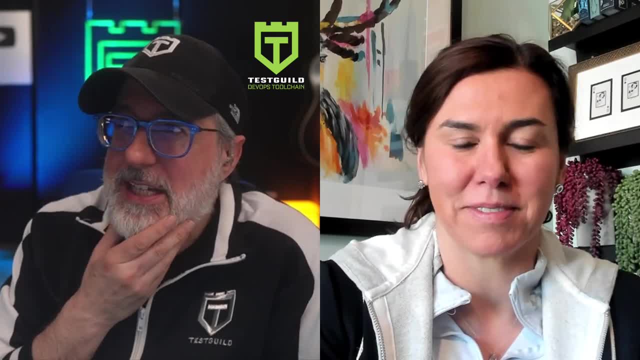 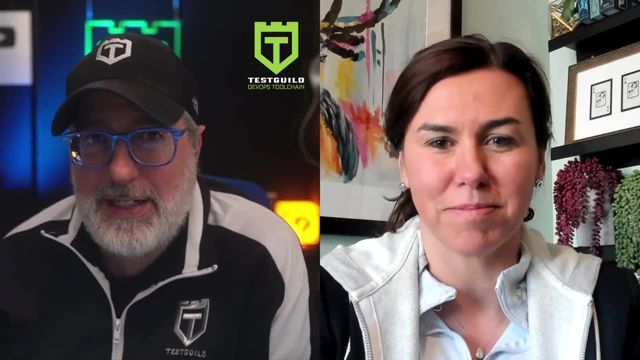 Awesome to have you. I guess, before we get into it, I'd like to maybe set the stage with defining some terms, just to make sure everyone's on the same page before. But again, I think it's a really great solution and a great technique. The first one is: I think we were 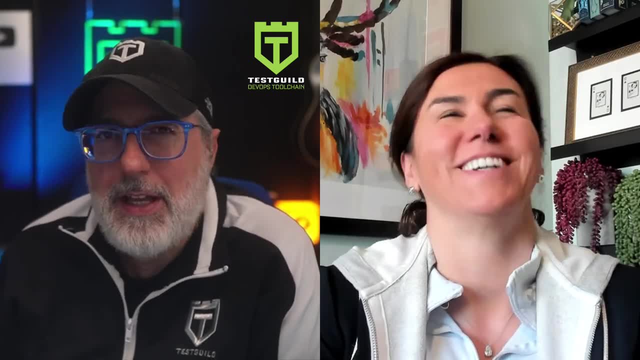 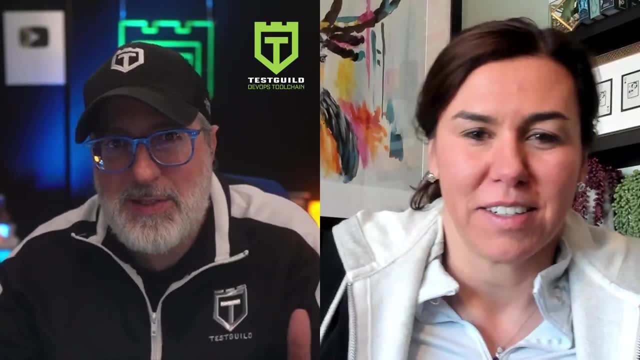 talking back and forth in email and you said you don't necessarily believe in DevSecOps- And this is a big debate. So can you tell us a little bit more like: what is DevOps, How does it compare to DevSecOps And why do you think Sec should be part of DevOps or not? 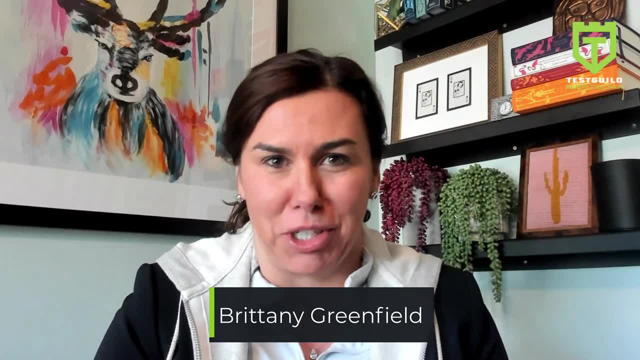 Yeah, no, absolutely. So. the reason I don't believe DevSecOps should exist as a term is it should just be DevOps, which should just be development. right, And if we think about where DevOps came from, it's a little bit of a different thing. It's a little bit of a different thing, It's a. it was really about breaking down silos, And DevSecOps is no different. The only difference is the job of the people that are responsible for delivering it, And what really happened was we had DevOps become, even if not fully implemented, but really the norm of development. by about 2015.. However, security was just sort of left behind in it for some very functional reasons. One: security, especially application security, is difficult, right? It doesn't run the exact same way DevOps processes do. There's a lot more. I call it sort of the system of checks and balances, like building a house. 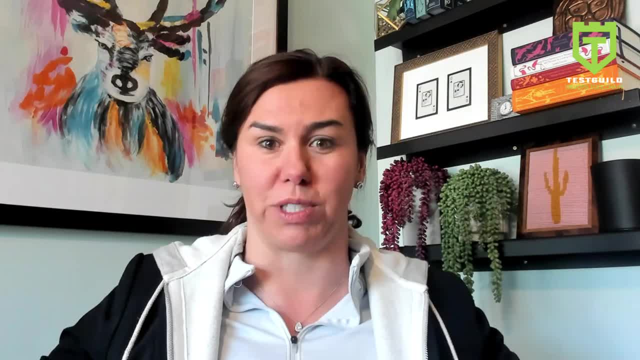 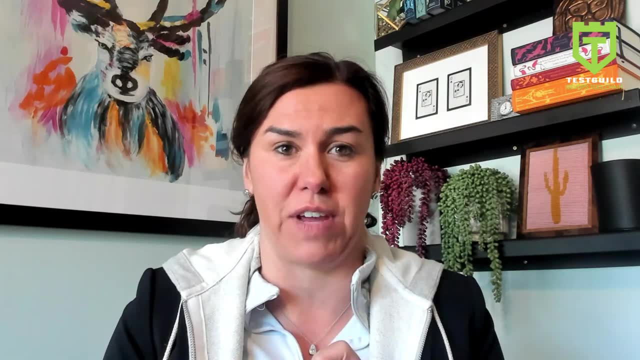 When you look at DevOps, you have that, you know, quality control to say, are there four walls and a door so I can call it a room? But security gets a little more nuanced in terms of the configurations and also the number of silos you have to break down. It's not just necessarily. just one security person you're dealing with right, Whereas you know one security team. you could also be getting as far out as legal and compliance and whatnot to be able to accept some of this risk, And so, really, that term- DevSecOps- was born. 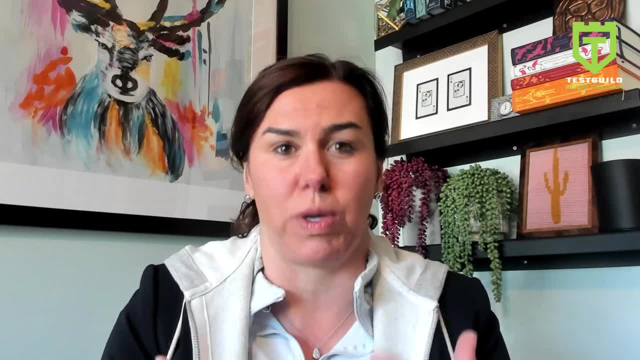 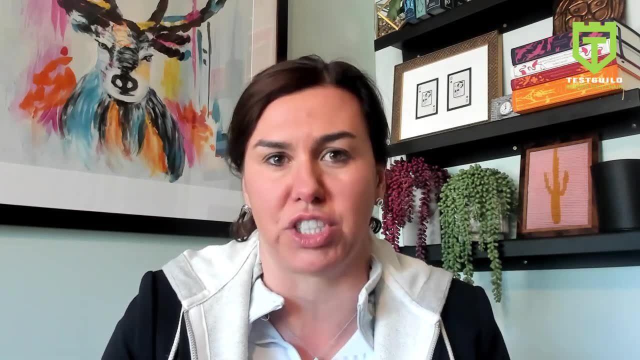 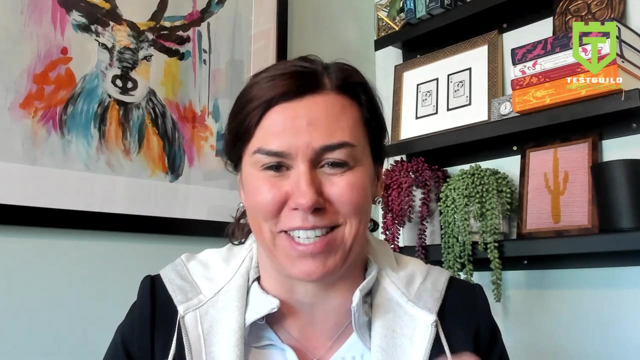 of the recognition that as development organizations we'd moved forward to say: let's break down silos, leveraging automation and orchestration to maximize efficiency on the team, And we hadn't brought security along on the ride. So you know, part of my mission with Wabi is to 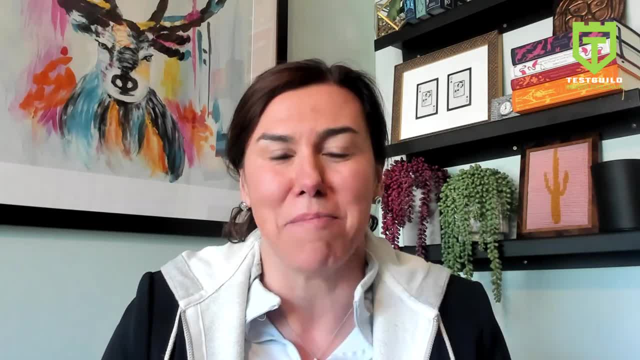 you know, break down silos, leverage automation and orchestration to maximize efficiency on the team. You know, make that term DevSecOps obsolete, because it should just be the norm. So how are you doing with that? You must speak with a lot of companies, a lot of users. 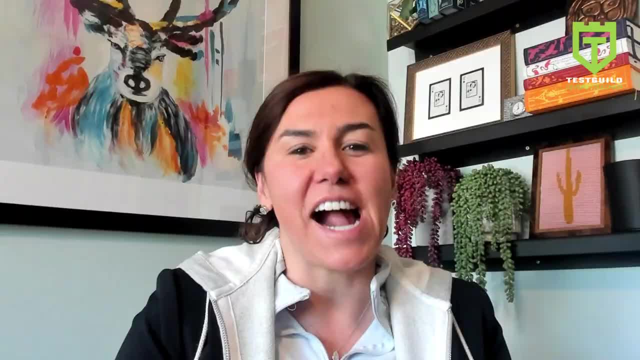 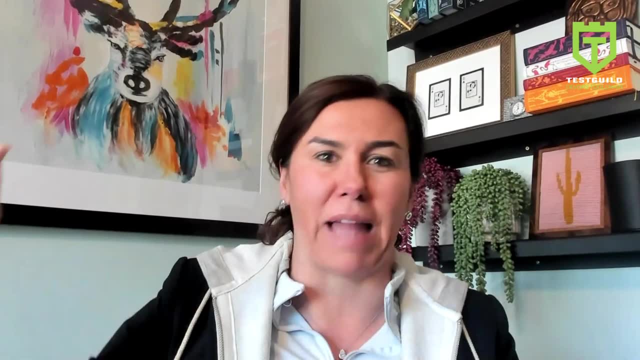 Are you seeing a breakthrough or is it still like a you know education? It is a breakthrough for sure, right, If you get into the sort of technical market adoption thing. it's in the plateau now, which doesn't mean it's gone away. It just means everybody recognizes. 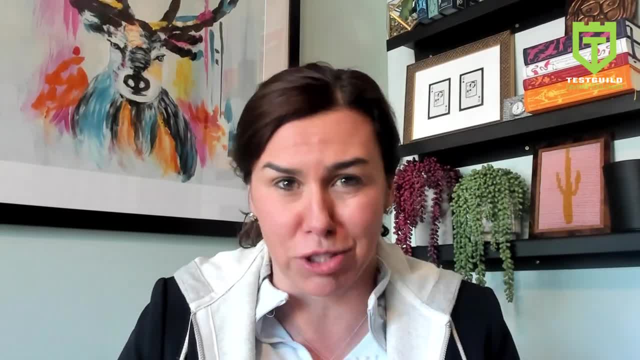 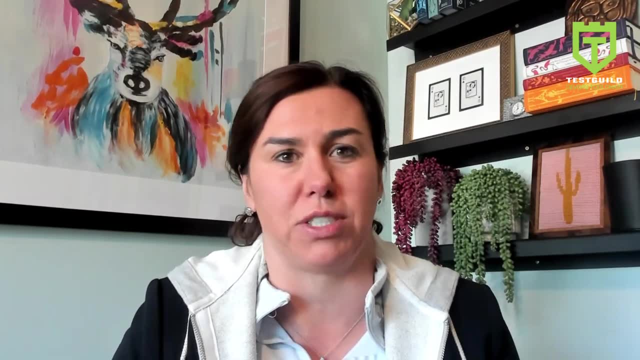 that DevSecOps is the norm Now, actually, from an execution perspective, it's not as good, And that's because it's no different right. The transformation to DevSecOps is not going to be any easier than the transformation from DevOps, other than the lessons that companies got to. 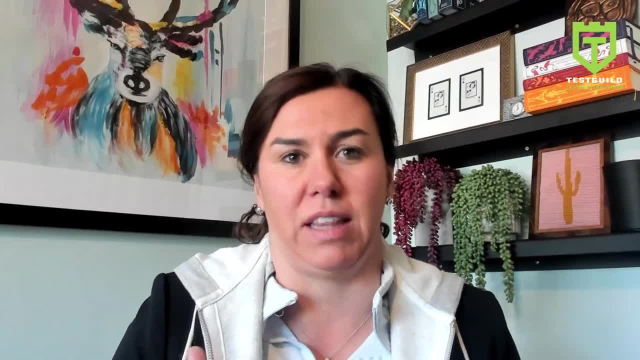 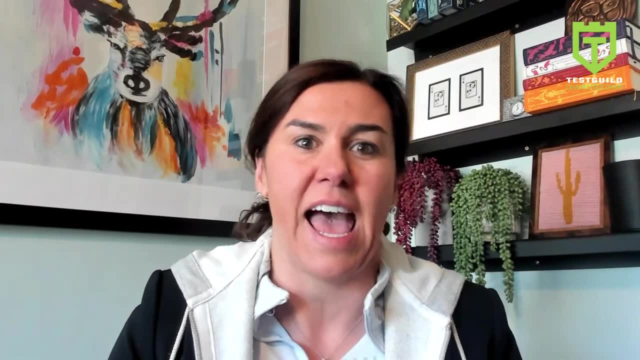 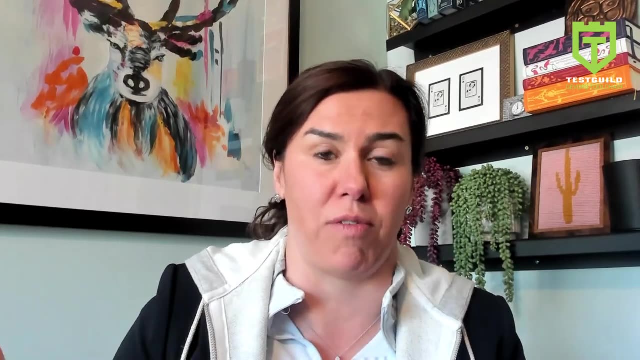 learn from that. And that's because we haven't leveraged automation and orchestration the same way in integrating security into the SDLC as we did in DevOps. And so now you compound that with the fact that 80% of organizations are actually true DevOps, And that's because we haven't leveraged. 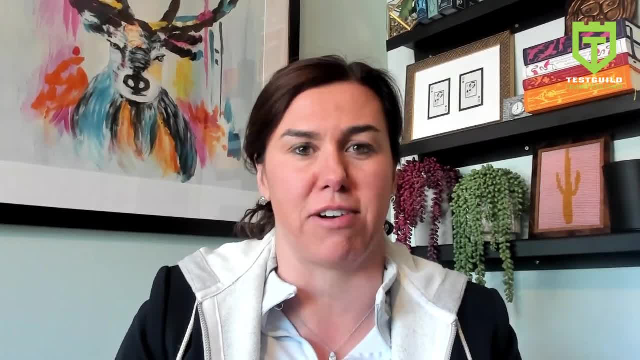 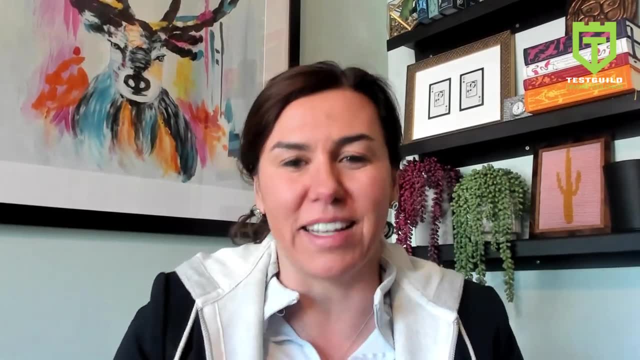 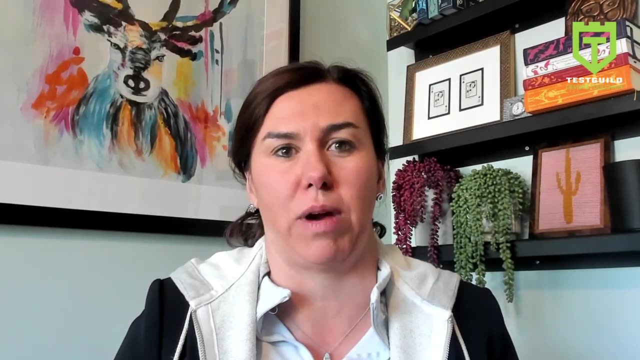 organizations versus having just sort of adopted pieces here and there, And all of these band-aided approaches are falling apart very quickly. So, yes, everybody knows this is the new norm for me, but most enterprises are actually still in the place where they've implemented DevSecOps. 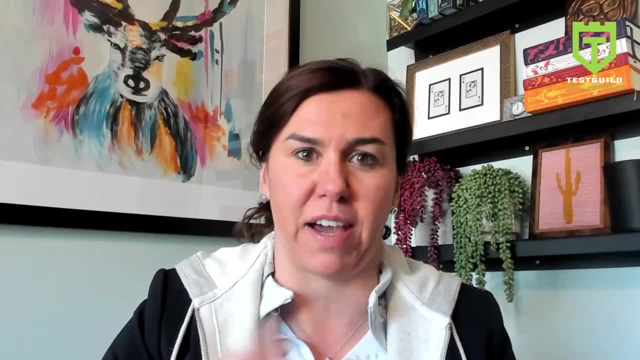 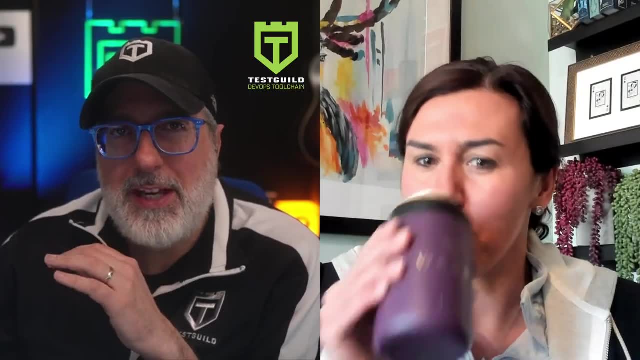 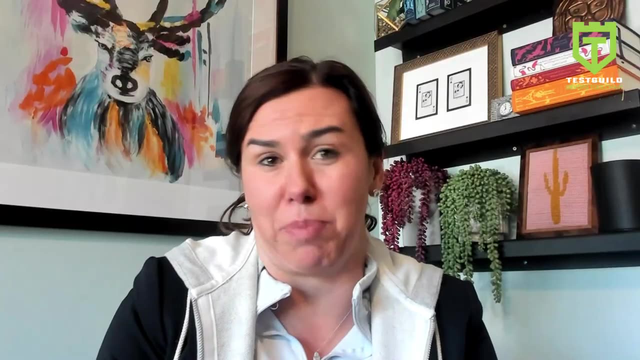 but they haven't codified it as part of their existing SDLC process. We can dive into why that is. Yeah, absolutely. You mentioned a lot of people on the execution piece, So how do you integrate then security in DevOps, Yes, Well, so that's our realm, right? That's what we call what has been termed application security. 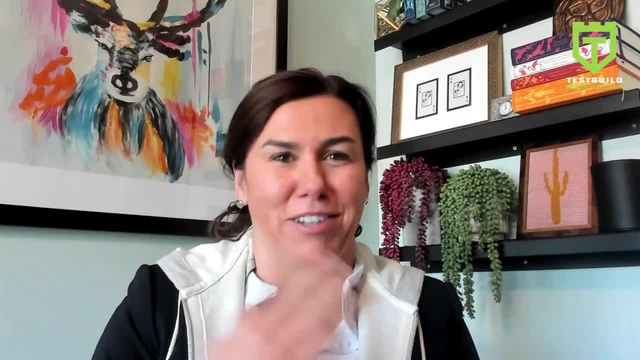 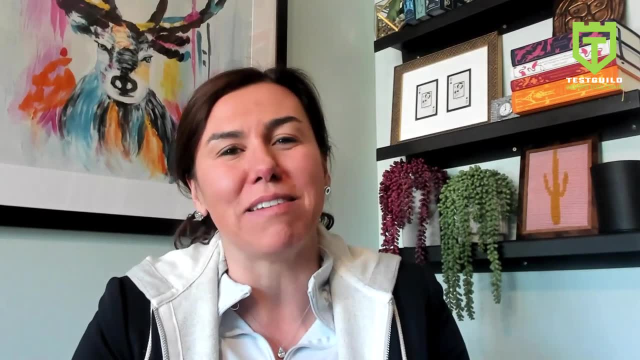 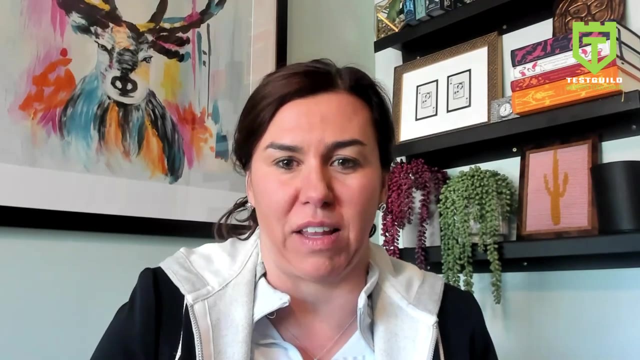 posture management, And so we're so thrilled that there's our own acronym in this big alphabet soup that security has and development has, And really what it gets at is none of the concepts should feel foreign to any development team right In development to make sure we get things out on. 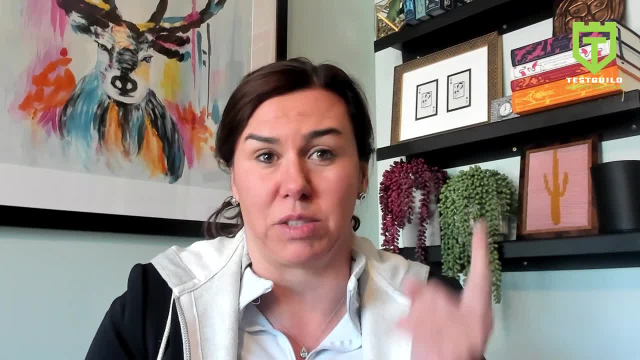 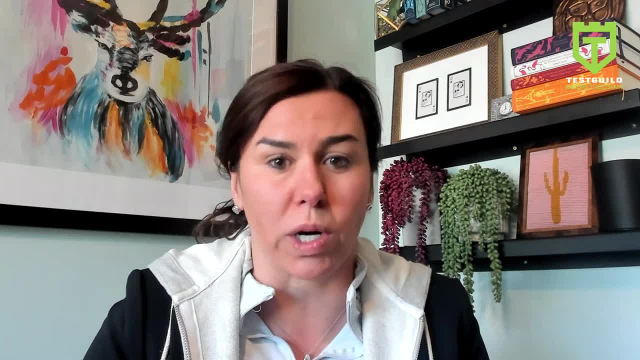 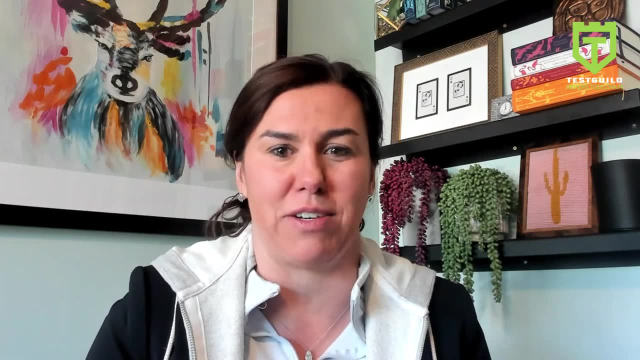 called vulnerability management, And we leverage orchestration right, Because that improves developer productivity right. We can't all be experts in the exact thing that we need to do now, nor can we be available at all the time, And so we need to know when we need to direct our attention. 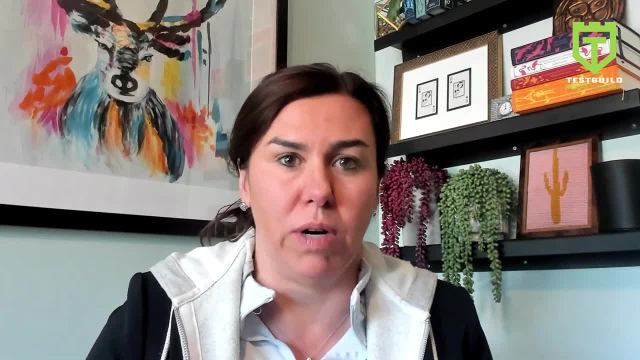 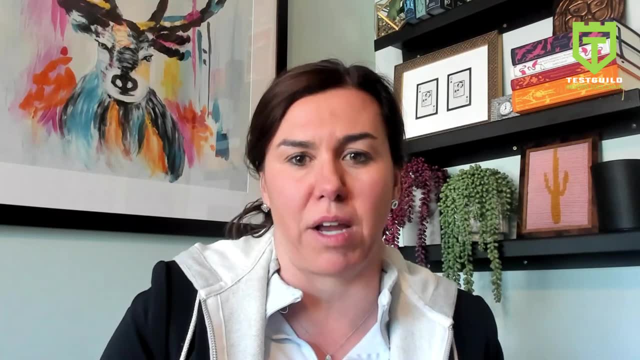 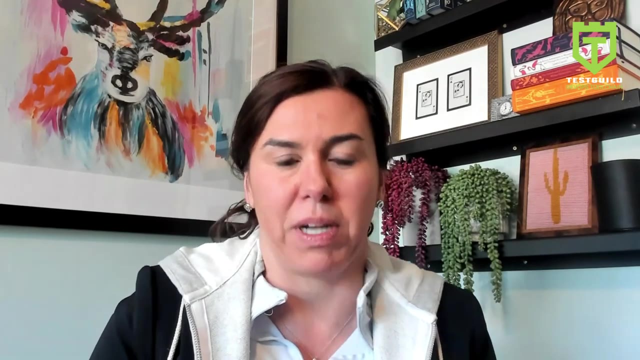 to something. And then the third is really what I think is the norm, now that we've seen, come with the transformations, isn't just monitoring but observability, And the analogy I like to use here is that we've created all of this data, but it's not enough to have data, You have to have actionable. 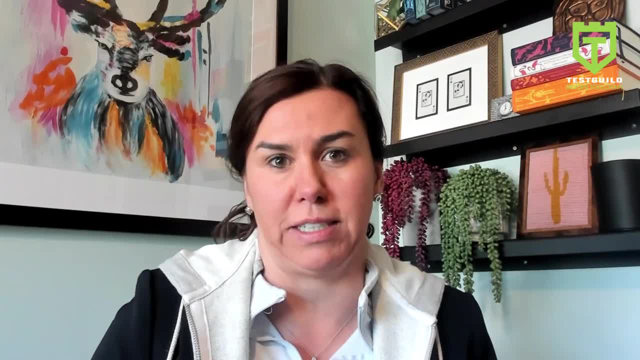 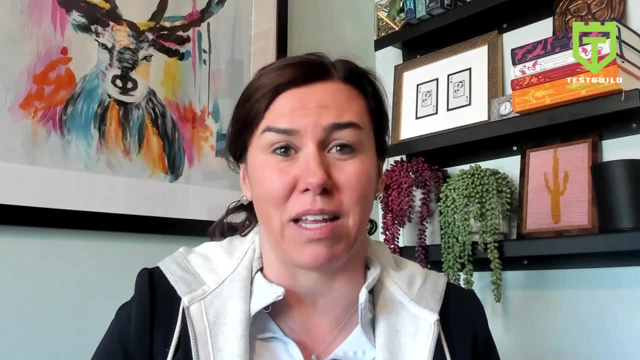 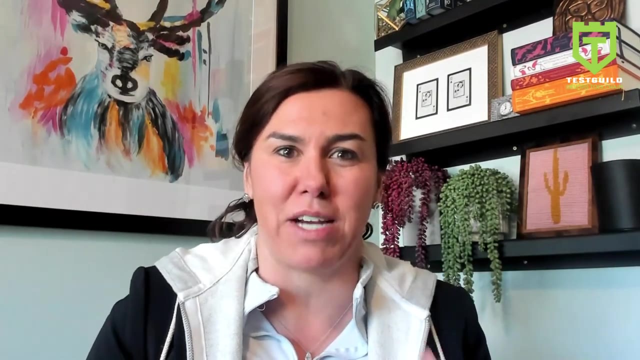 information Data is saying: hey, it's 34 degrees. Well, here I am in Colorado, and that is a warm day here, beautiful spring day. If you said that to somebody in Los Angeles, they'd be pulling out the puffer jackets right. Maybe even apocalyptic, And that's where. that's the information part. 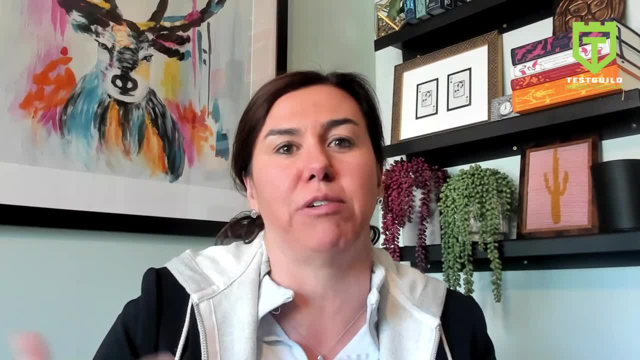 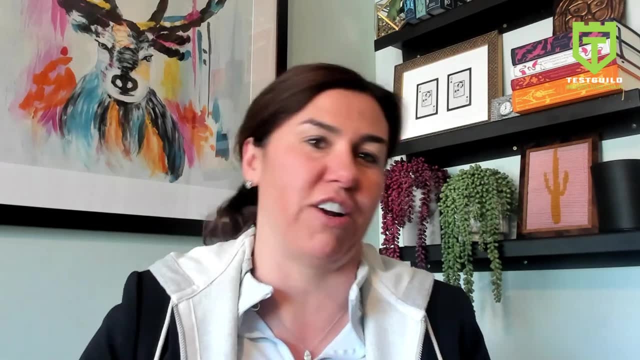 because that information is going to provide the context that allows you to make educated decisions, And this is really the area we address. that doesn't say: hey, security, can you suddenly start acting like development? And hey, development, can you start to act like security? 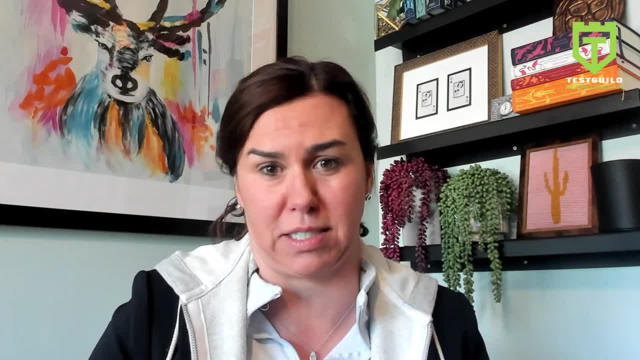 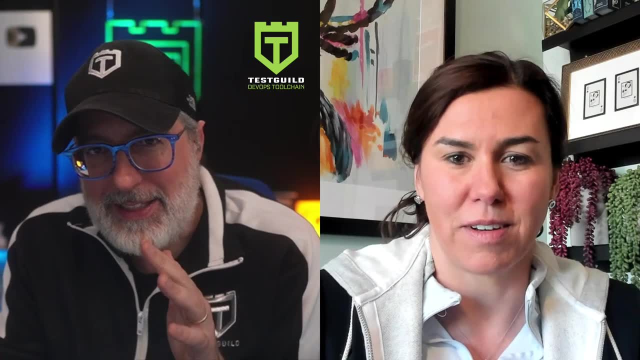 Let's use everything that's already available to us to marry the processes. All right, Let's dive a little more into that then. What is Wabi then? I mean, is this AI Like AI? we have all this data, so we'll throw some machine learning and all of a. 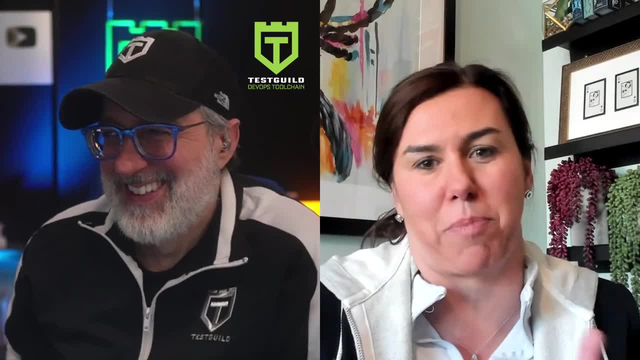 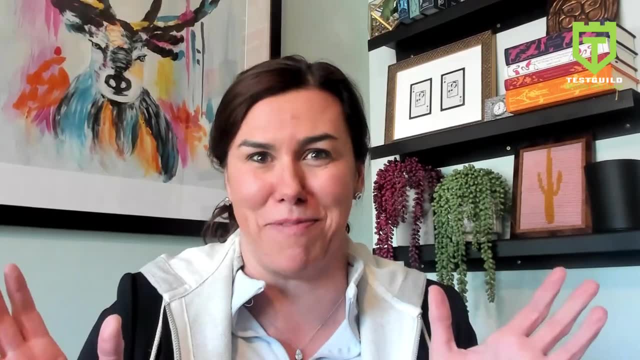 sudden security posture management. like: how does this work? So AI is an intrinsic part of it, right? Cyber has always been rife for AI applications, even before AI was at the tip of everybody's tongue Because of all the data, right What? 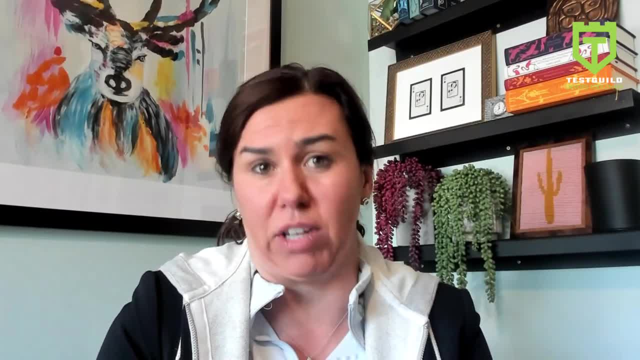 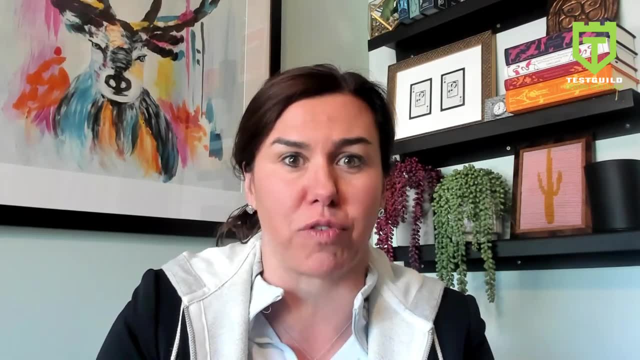 we want to do, and especially in cyber. there's a real scale issue- And this has been one of the challenges in DevSecOps programs- If there's one application security manager for every 100 developers. So we've done some research ourselves that actually shows. 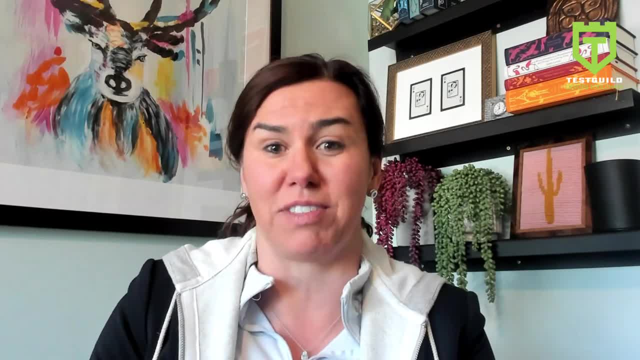 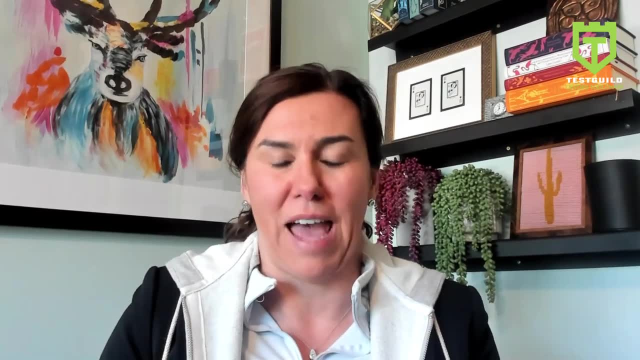 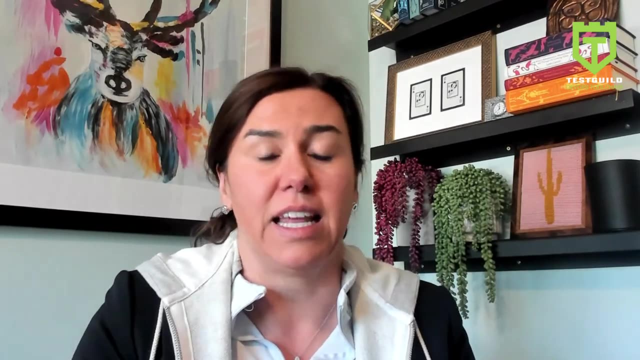 developers recognize that security is responsive to feedback, but they don't have those automated feedback loops. So how can you be responsive if you can't get back in real time at the same pace? right, It's just. this is one of the many areas of disconnect, And this is where AI is super. 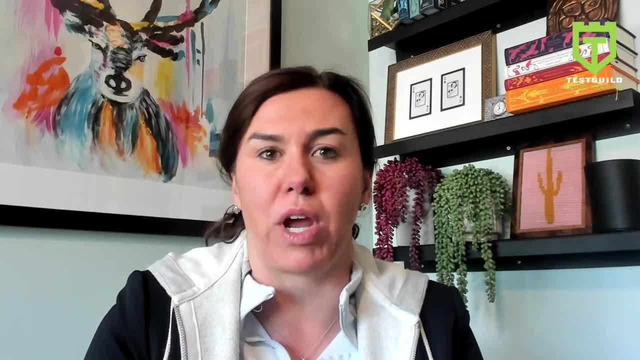 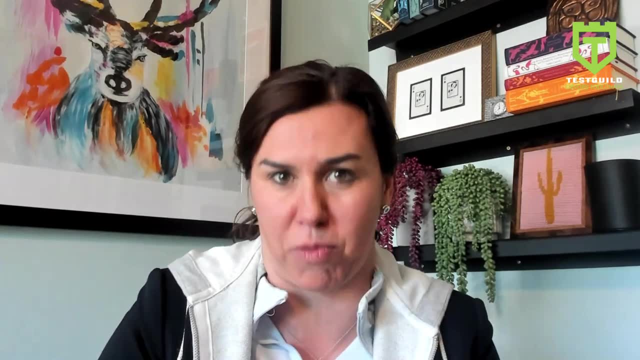 helpful. It's an intrinsic part of our platform, But what we are is a SaaS platform that orchestrates the end-to-end application security lifecycle as part of the software development lifecycle. So developers get to keep doing what they're doing, which is developing code, and they get 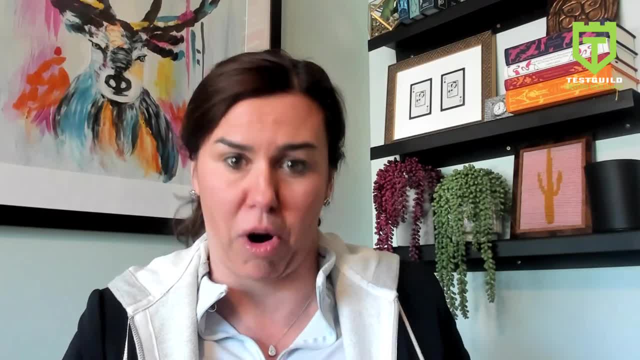 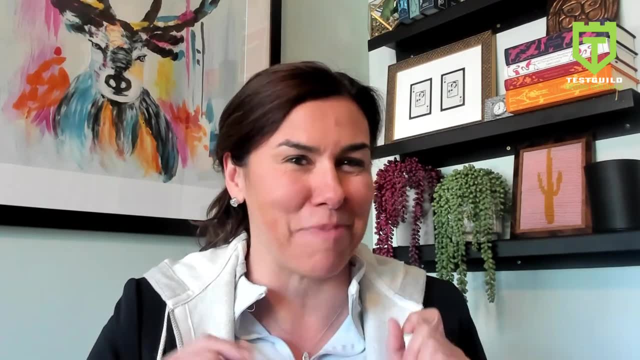 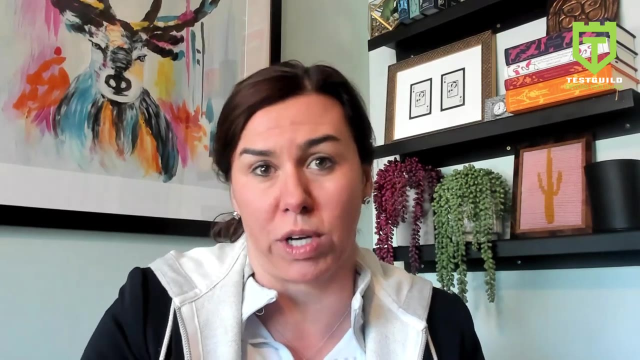 the security tasks that they need to fed into their process at the right time. So, rather than, hey, we're going to stick you in security training once a quarter and expect you to magically remember the right security thing to do in exactly this right time, we're going to orchestrate that. 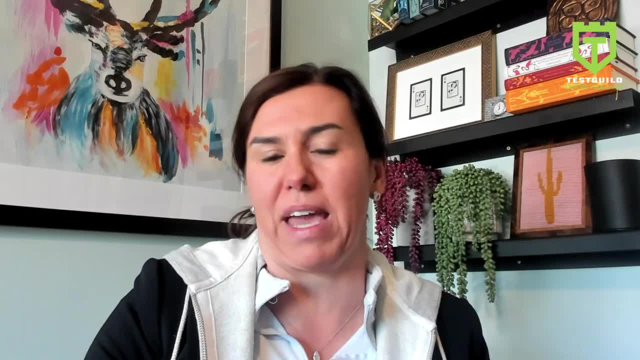 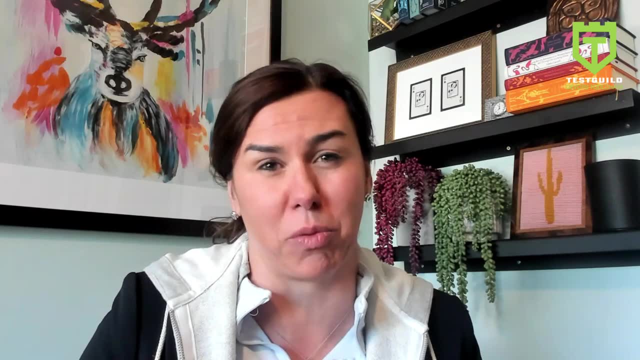 and sometimes do that for you or just tell you what the manual step is and then allow you to have the chance to do it. So that's what we're doing, So we're going to orchestrate that and put that feedback in. So one of the things I think every developer has become very familiar with. 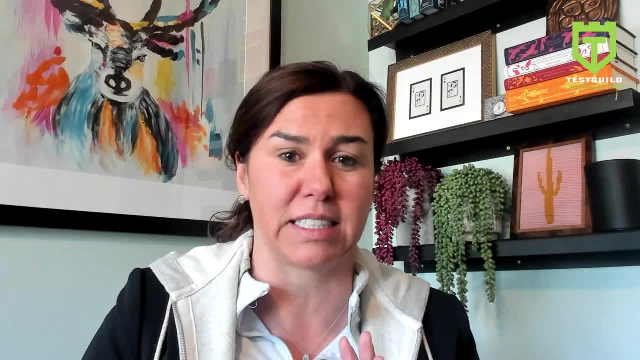 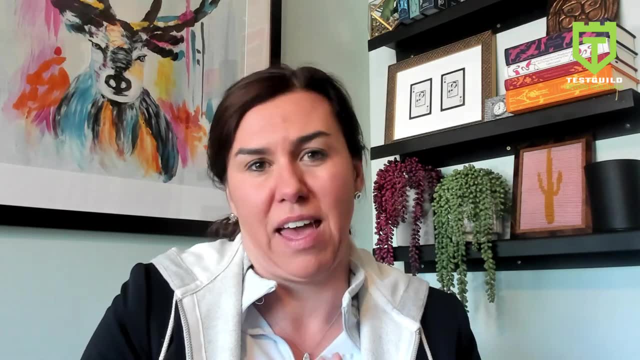 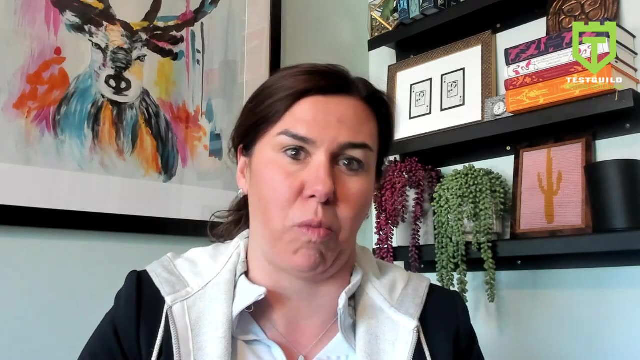 nowadays is SaaS, scanning, static analysis, And that's something that many of our customers require to be completed before the PR. So, as a developer, instead of having to hit a button or call your friendly security person, Wabi, once you submit, the PR will automatically kick that off. 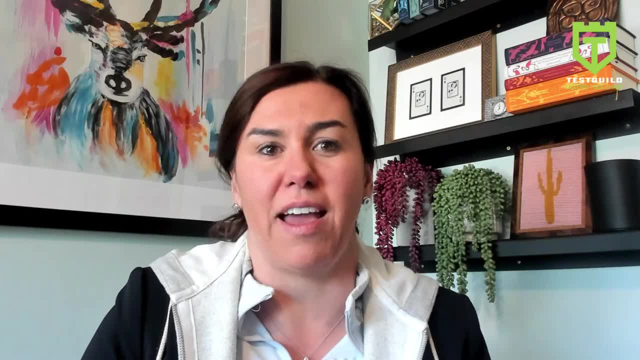 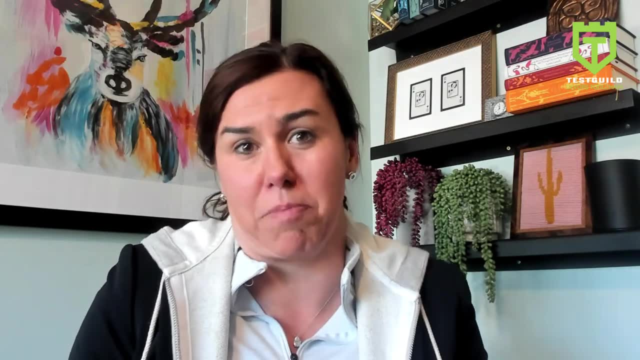 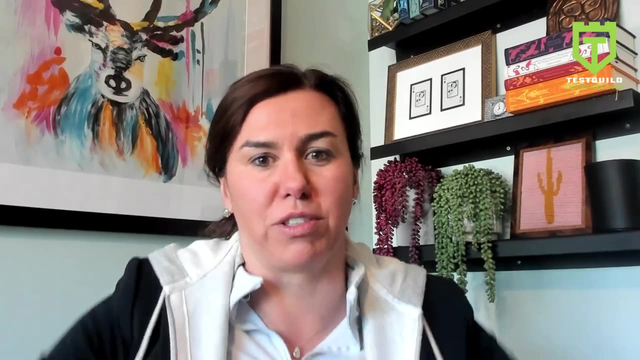 bring those results back and prioritize them for you. And if your company says you have to fix the rules first- kind of like bugs- we're going to block you from completing the PR or allow you to route it to somebody for an acceptance. That's one example of that, But that goes from the design. 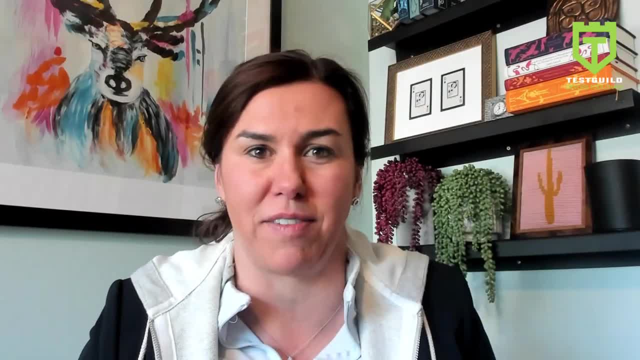 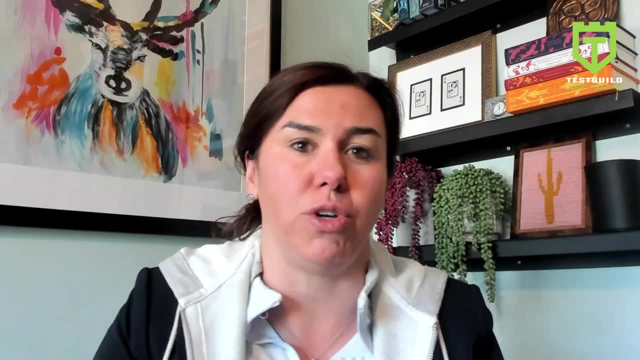 perspective right. Some customers even have, depending on the kind of confidential information. hey, we've got to have an actual meeting before we'll even release the features. We can orchestrate that to also the thing I think we don't talk about so often. we talk about the 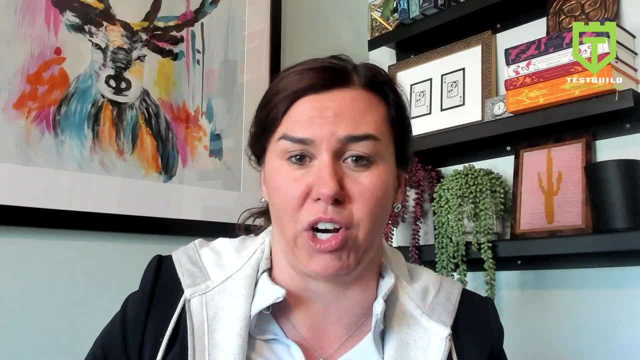 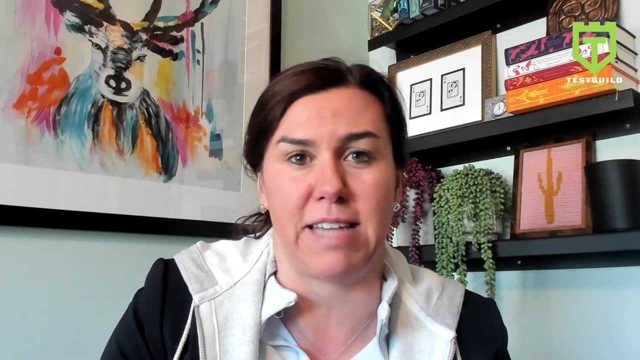 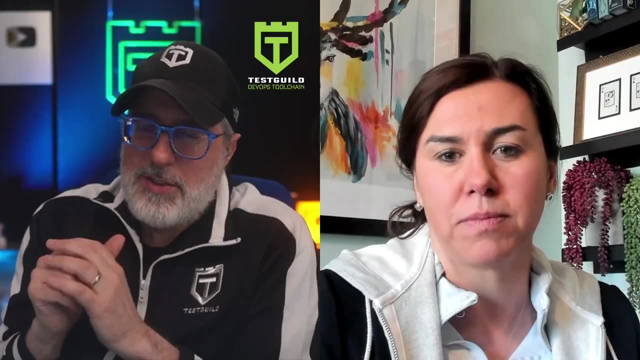 differences between security and development, but not the similarities. Both security and software are living, breathing things, So changes are happening all the time. So we can take in changes from the security side or from the application side that may change the security requirements, All right. So how is this information fed? A lot of people I think they know of like a 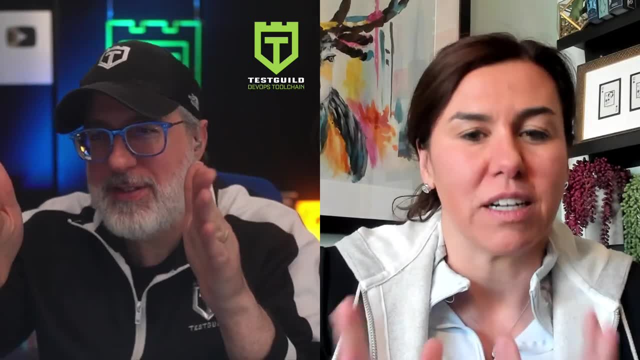 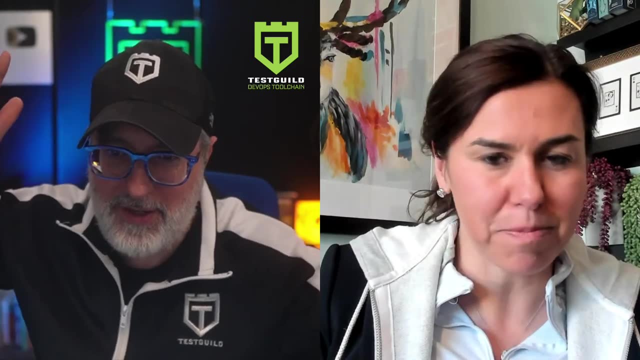 security scan. You check in code, you do a security scan. That's the first stage of your pipeline. Didn't pass, doesn't get changed. You check in. This sounds more like an end-to-end kind of shift left, shift right. How does it feed? 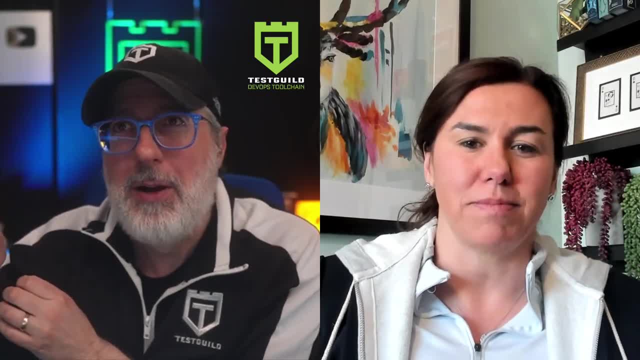 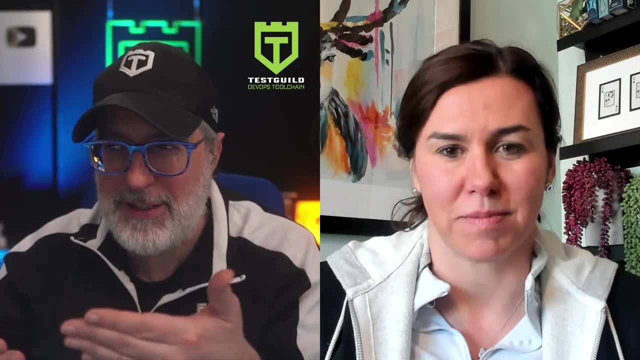 the information? How do people get the information at the right stage And not being necessarily security experts, when they do get like, hey, this is an issue like, how do they even know how to fix it? I don't know if that's a lot of questions wrapped in one. 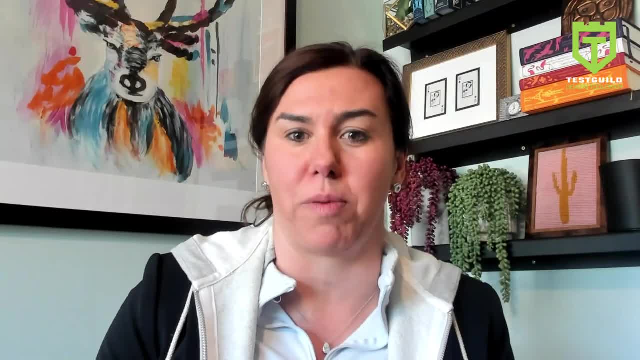 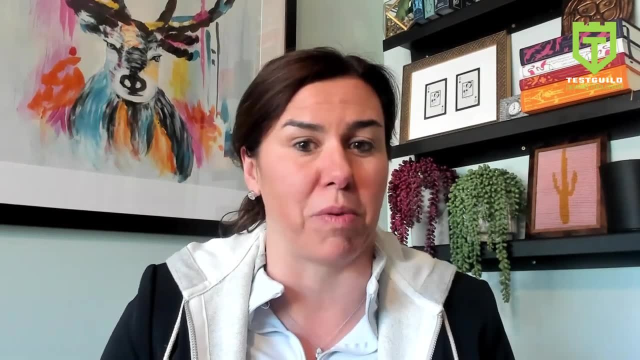 No, no, no, no, But you hit the nail on the head. This is why this has been so complex and what's made Wabi really a pioneer in it. So let me take a step back, because I used a phrase that most people 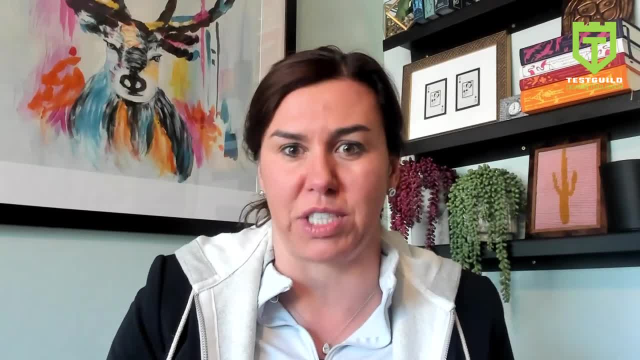 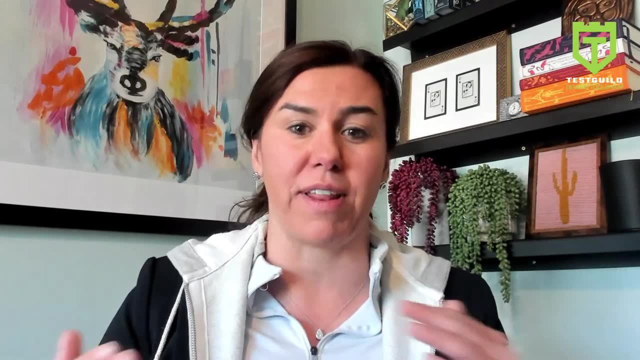 might not be familiar with. We're all familiar with SDLC right, The software development life cycle. Application security is no different. There's an application security life cycle, different things, It's not just the testing. This is where, I would say, the fallacy of DevSecOps was. 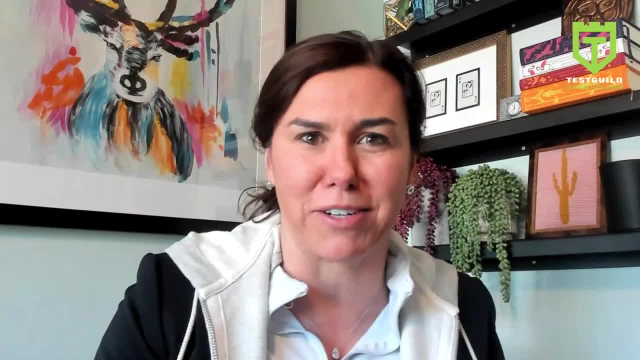 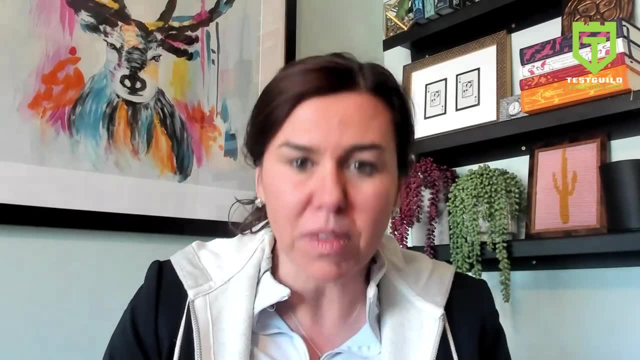 that: hey, you've got a DevOps tool, I've got a tool to secure it, And now we're doing DevSecOps. right, All that did was create more data without information. So the application security life cycle really looks at it at the development of the product. 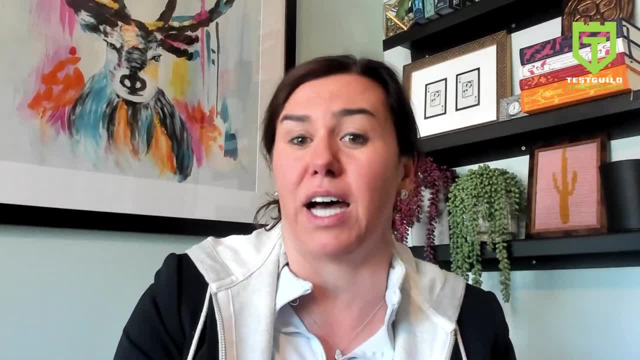 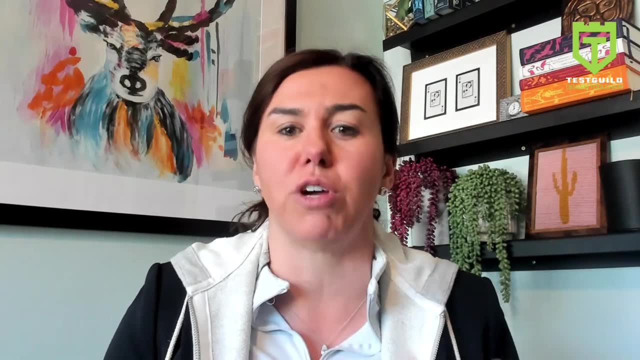 and says: what is the thing that has to be done at the right time, And it's not just testing. A lot of times I'm sure folks in your audience are familiar with the term secure coding. There's no test for that right. We just need to say, hey, you're dealing with PII, So you need. 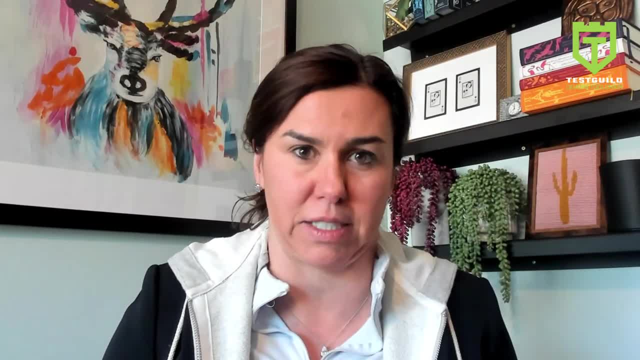 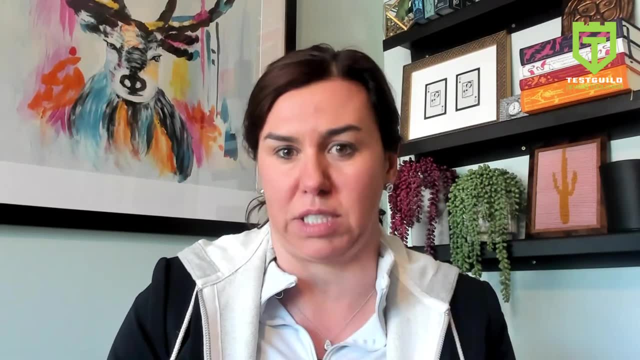 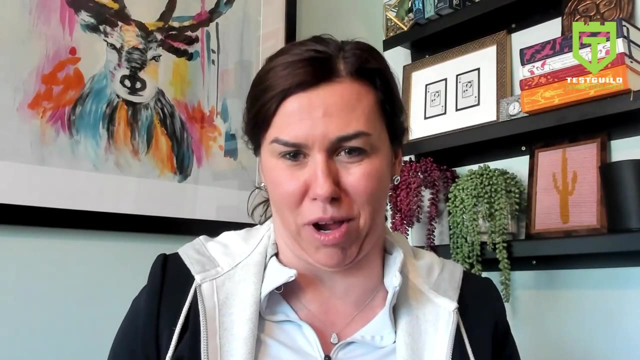 to put a 15 minute timeout on. That's just a best practice. Or there could be gates that are put in the right time, But in the singular of a policy not being followed, it would be fine. But maybe you have 20 policies that weren't followed across an entire team or product, And that's when security 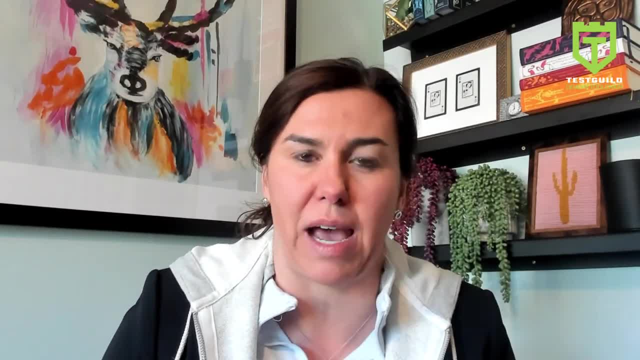 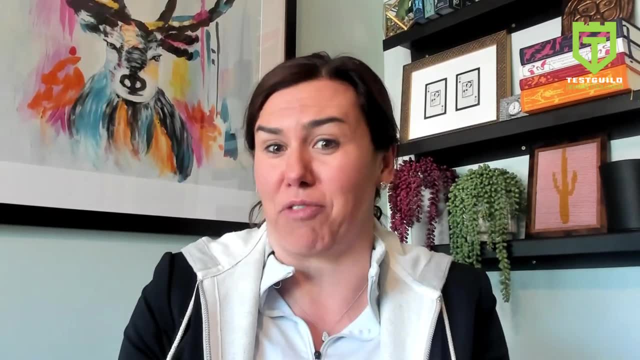 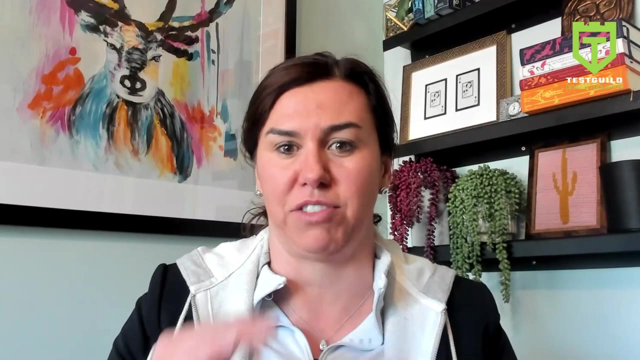 would want to stop it, And so when we talk about the application security life cycle, I'll use a simple analogy. Something that we all share is that we go into buildings every day- right, And we trust that we go into those buildings every day and they're safe because the right set of checks. 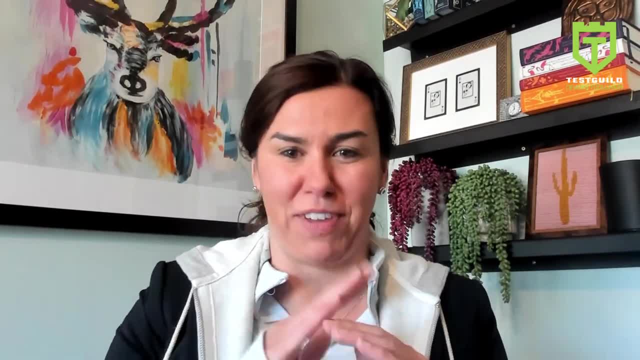 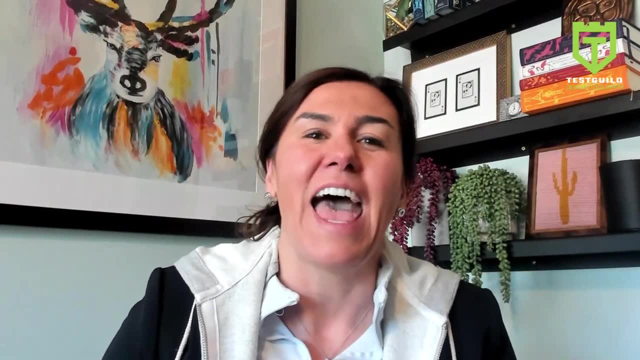 and balances has been applied And we trust that. we go into those buildings every day and they're applied, And when something needs to get fixed, it also gets put onto a punch list- Should start feeling very DevOps-y right. This is the world of application security, And so that's when we talk. 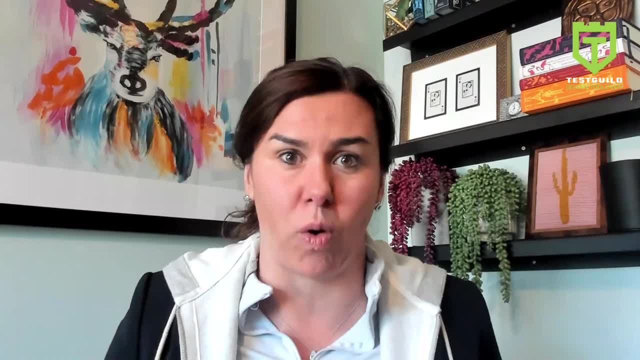 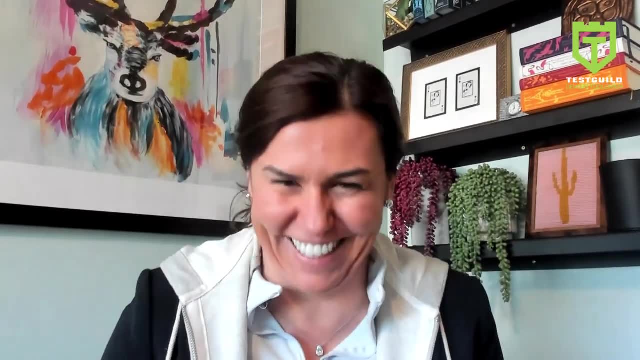 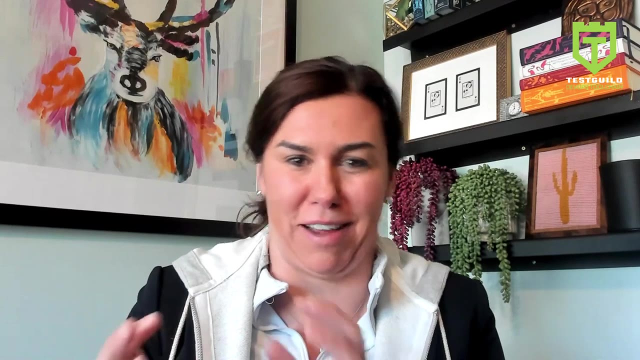 about that end-to-end. And what Wabi does is we manage that whole set of checks and balances And on top of it, as we know, in development nothing ever goes to plan right. Software isn't perfect, So when something doesn't go to plan, we also manage that set of chutes and ladders. 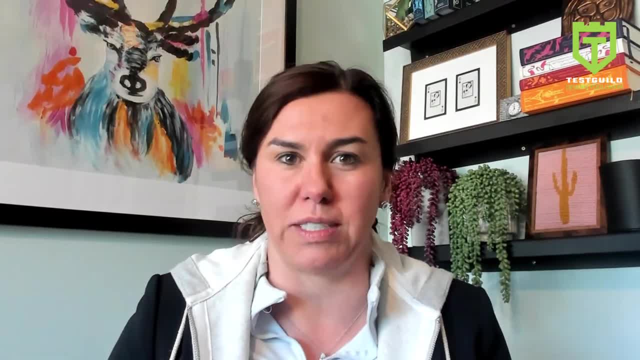 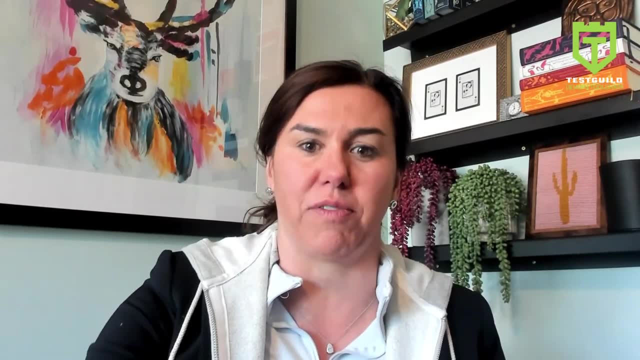 so to speak, And that's when we talk about that end-to-end and what Wabi does is we manage that of where it needs to get routed. So organizations, just like the way we, make educated decisions about what's good enough to ship today from a quality perspective and from a future perspective. 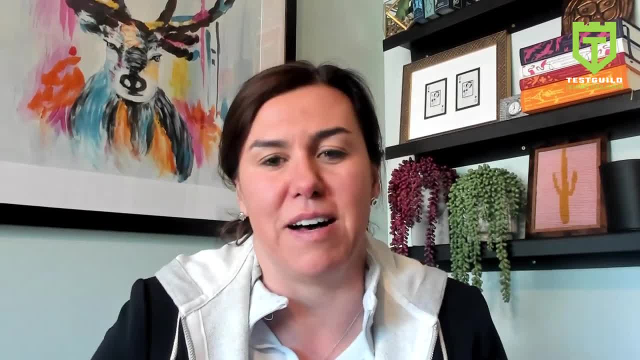 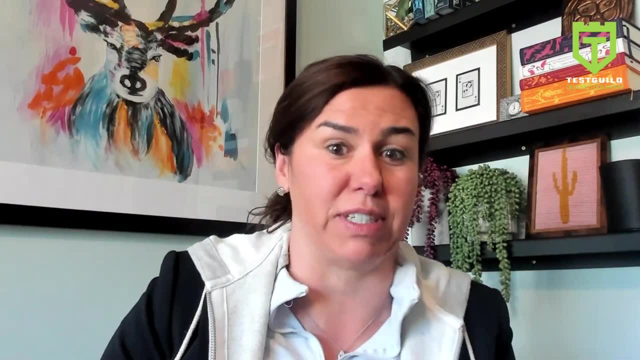 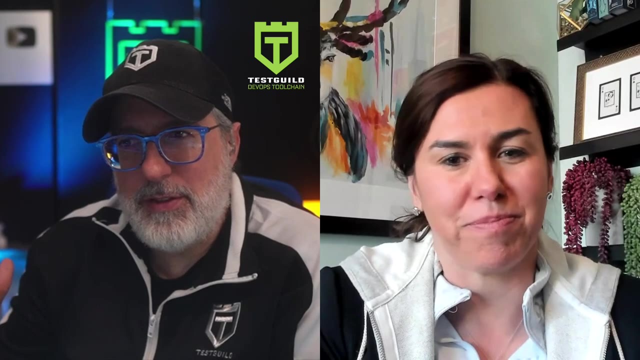 can also do that from a security perspective. So that's when we talk about that application lifecycle. It marries exactly to the SDLC. It's just a different set of rules, Gotcha. So is it like a compliance application then, where each company may have different? 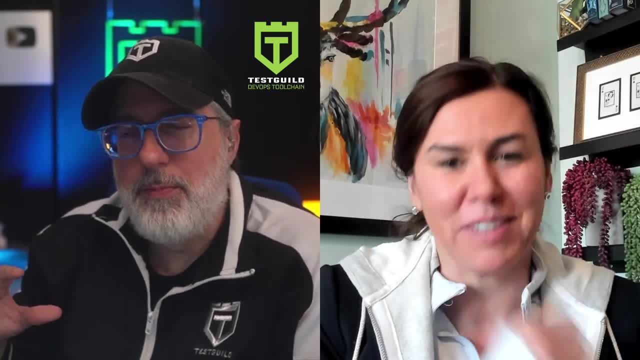 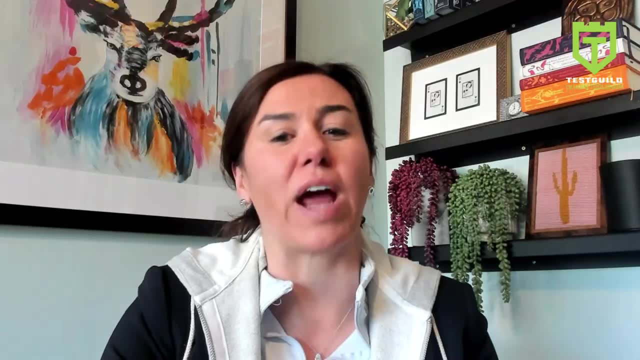 standards that they want to apply to, Or is it just a set of rules That they want to follow and you would merge, they would put it into the application and that would manage then compliance as well. Correct, You've hit on a couple. 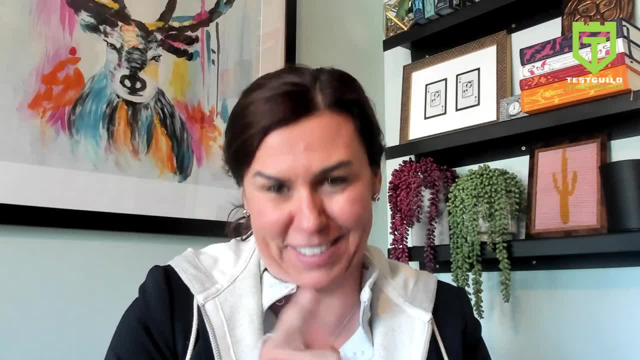 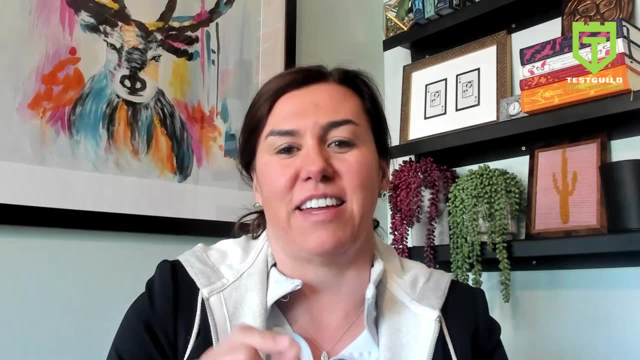 three very important points. So I'm going to pick on the word compliance, because compliance is a dirty word. If you're only doing security to do compliance, then you're just doing check the box, security, right And security. but you redeemed yourself. 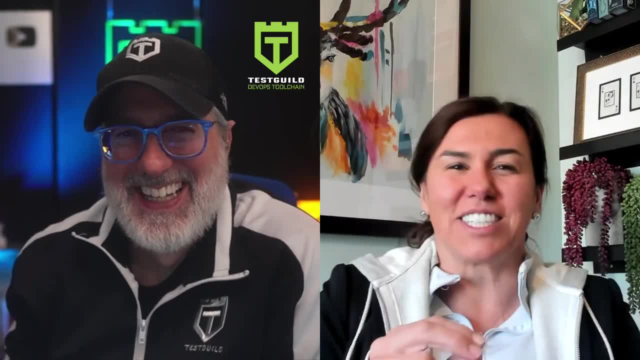 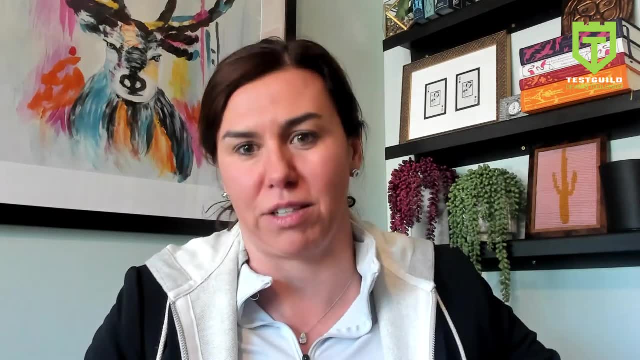 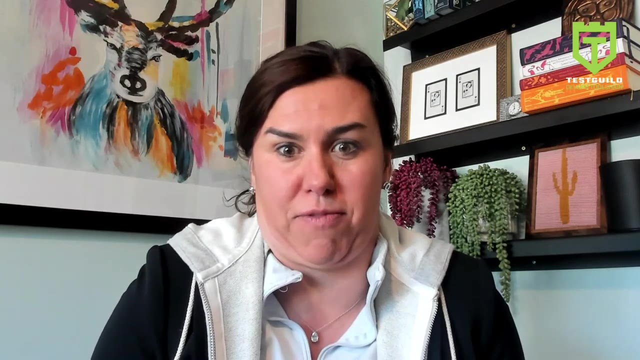 in the next statement, Right, Which was: every company has their different set of standards, right? And those standards are obviously sometimes driven by regulatory standards or frameworks that they choose to, But the way a company chooses to implement that standard is different, right, Those standards? 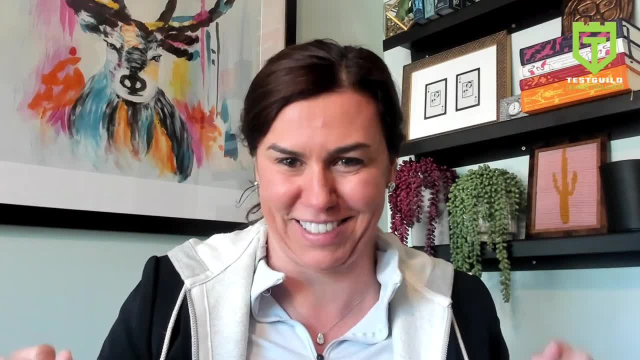 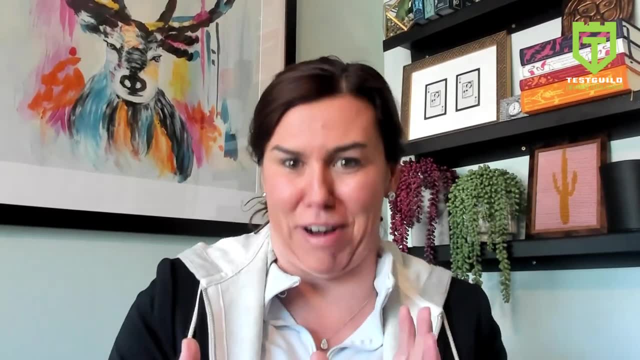 say something like: use a firewall and check it on a regular basis. And, just like humans, your risk profile and my risk profile are different, Regular is different, And so that's. that gets us to the point where we're like: okay, I'm going to do this, I'm going to do this, I'm going to do this. It gets to that nuance And sort of. the third point on that is that each company, especially in large enterprises, treat also their applications with different risk. right, If I'm a bank, you know to the end user. an end user sees bill pay and wire transfers as the same thing. 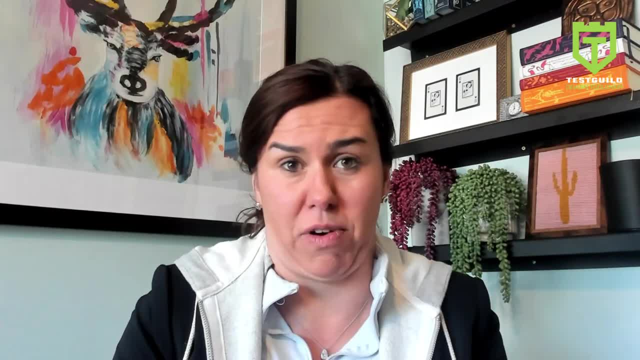 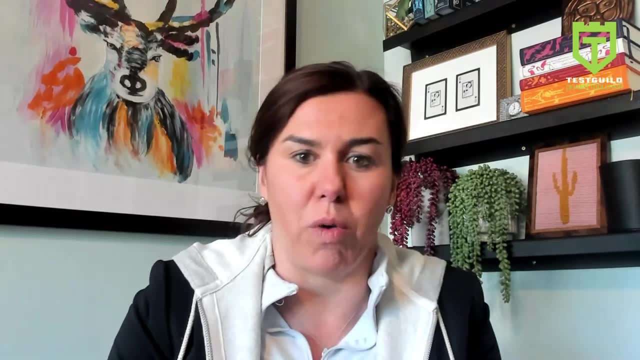 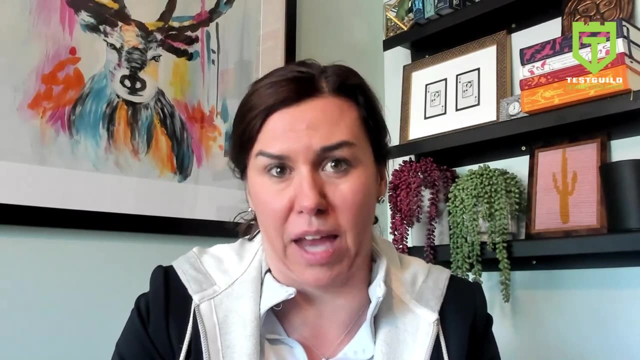 I'm sending money to somebody, The bank sees that very differently, even if nothing else, because the wire transfer platform is separately regulated. But you know also, wires are instantaneous, Bill pay is batched. So as you start to think about the world of risk that you're willing to accept on that, 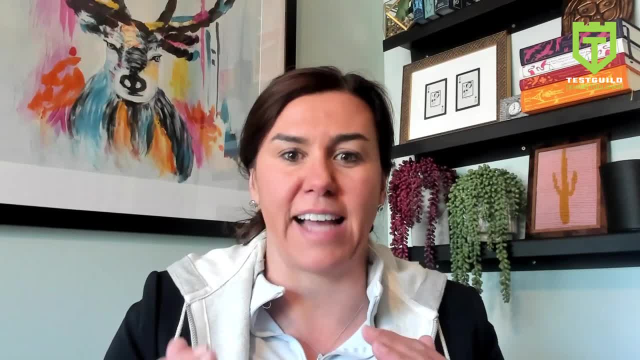 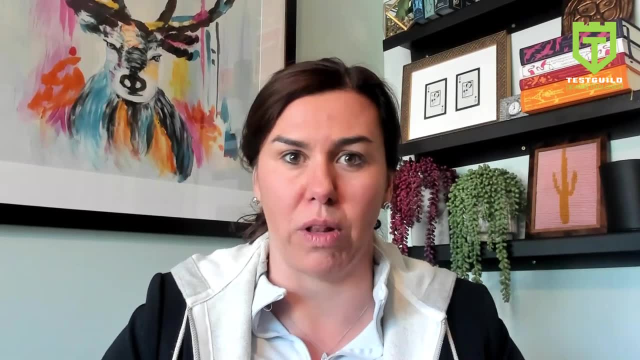 you're going to implement those standards differently, And that's why this gets very nuanced very, very quickly As we think about the ways that are. you know, a lot of times, security is thinking about how the outside world is trying to get in. 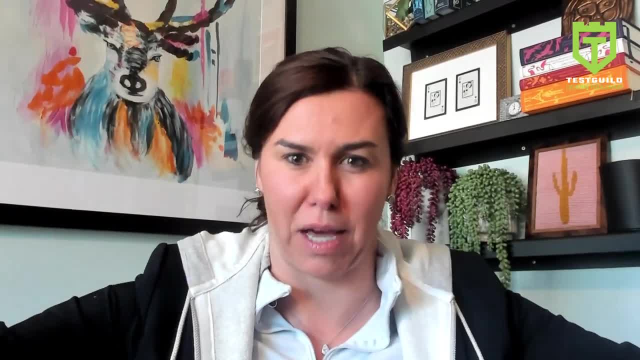 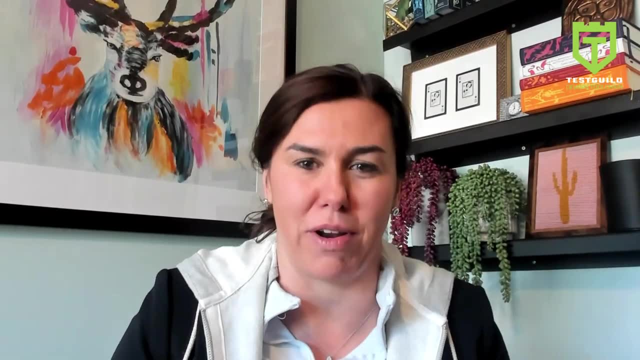 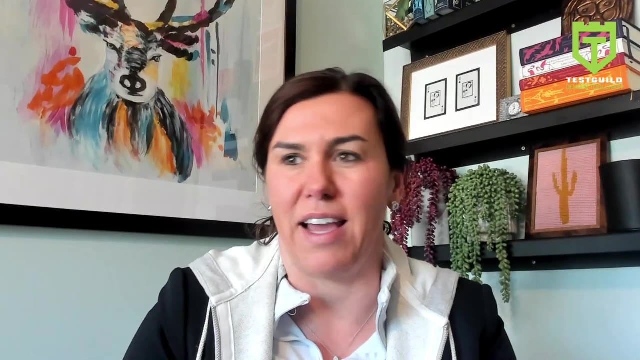 right And what our risk profile is on the outside world. and development really aligns with the business, customer promise, delivery risk. So how do you marry those two? So that's why I say compliance is a dirty word, because you're not thinking about business risk and customer risk. 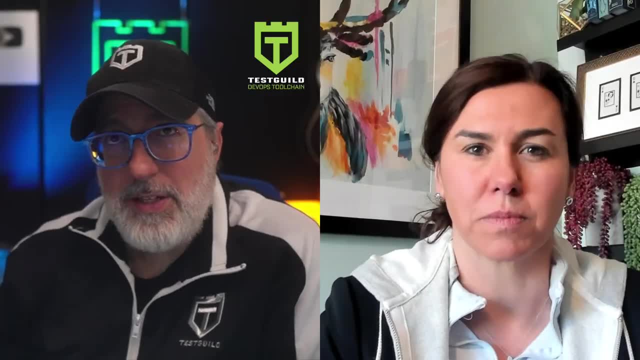 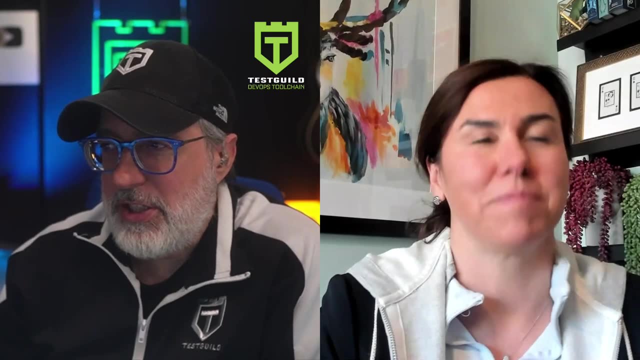 if you only think about compliance, Right, right, So I used to work for a healthcare company and they would sell radiology machines to different regions, different countries, and they all have their different regulations And you know, we could be audited by the FDA. So it sounds like. 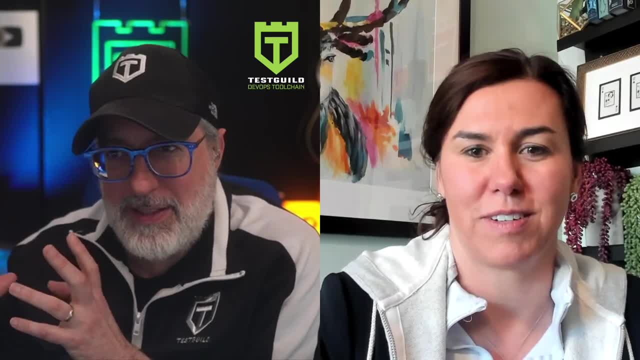 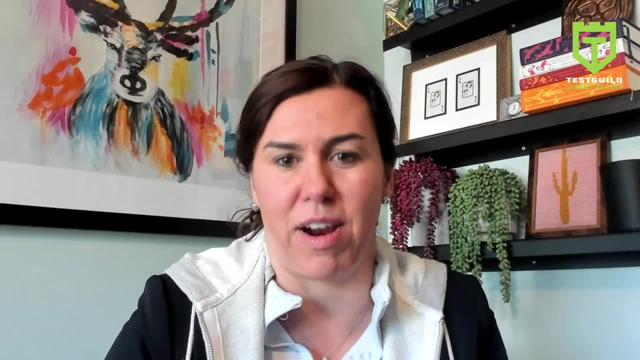 having a tool like this would help Automate that process, rather than having like a checklist that could kind of evolve with you as well as regulations change also. Exactly right, The world that we're living in is very dynamic, So changes are going to happen. 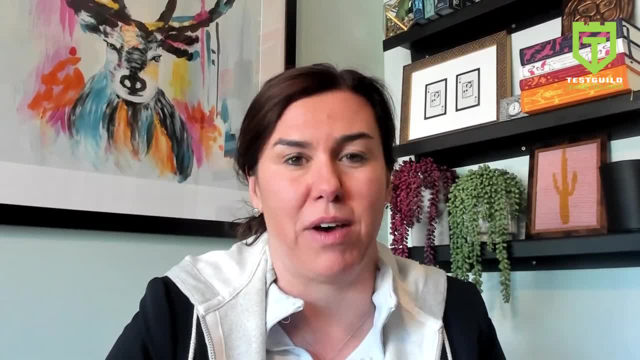 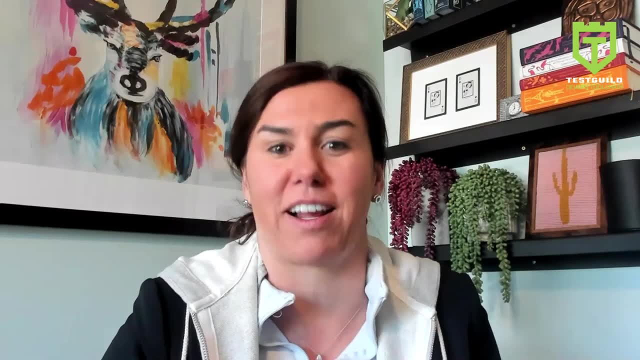 And you know that checklist this is. you know you asked earlier about the reality of DevSecOps having been adopted. This is how people are doing application security by checklist now And you want to know what happens. Security calls development and they go. 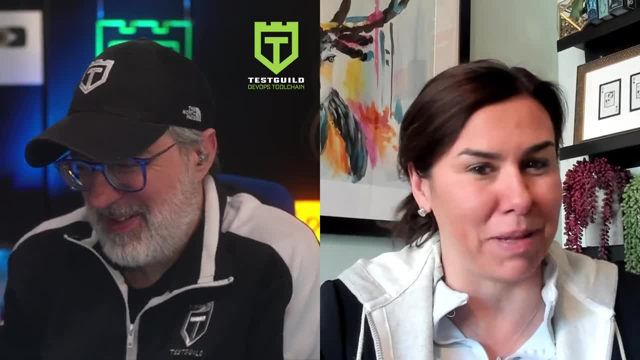 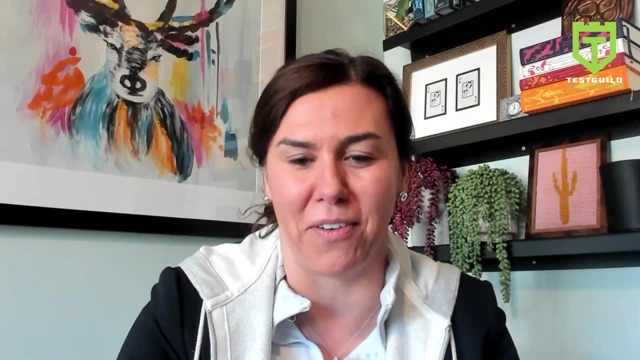 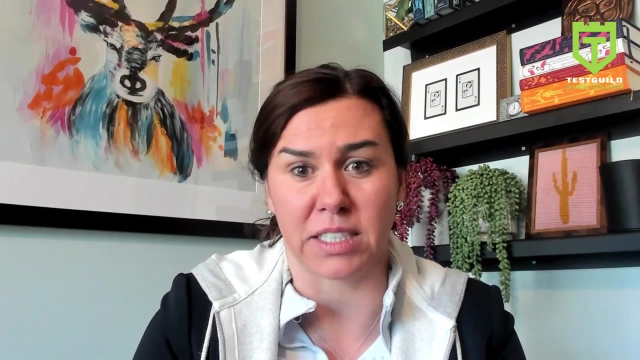 hey, did you do that thing I asked you to do, Which was probably a month ago? Yeah, of course, Right, We have. we worked with one large telco said: look, we accept the fact that nine out of 10 times we give development the pass because we. 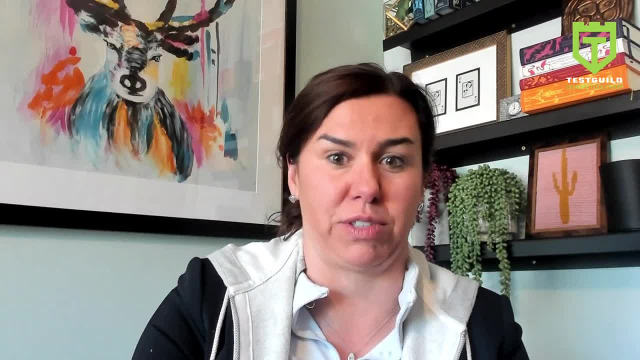 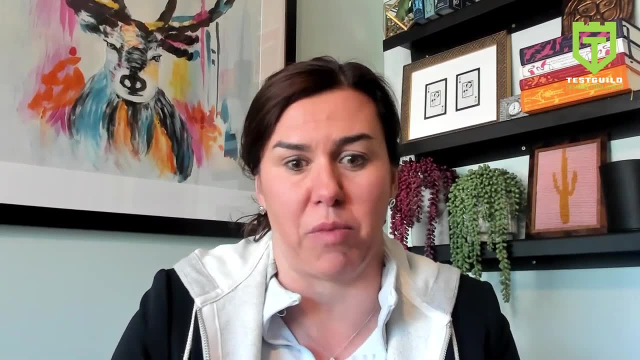 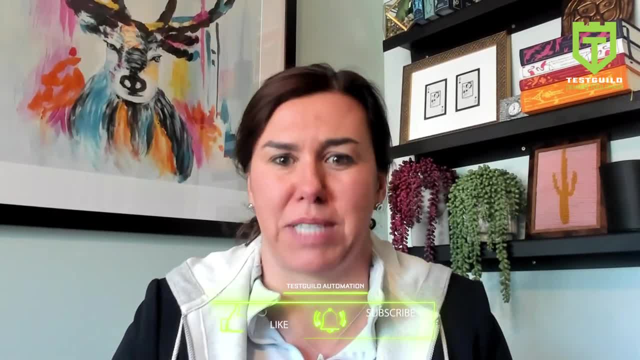 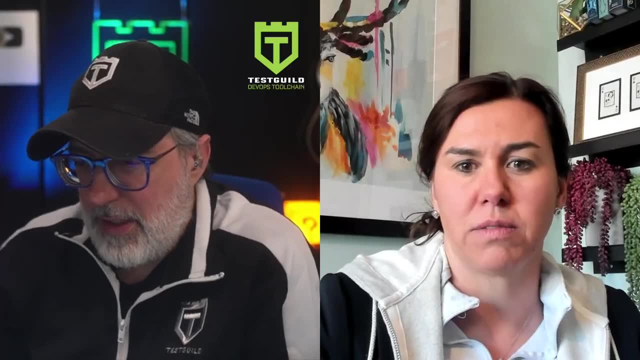 Again. this should all feel very familiar. This was the same challenge Dev and Ops had at the very beginning. that was, creating a drag on actually delivering the product. Love it? Yeah, I know a lot of developers have a large definition of done like security. 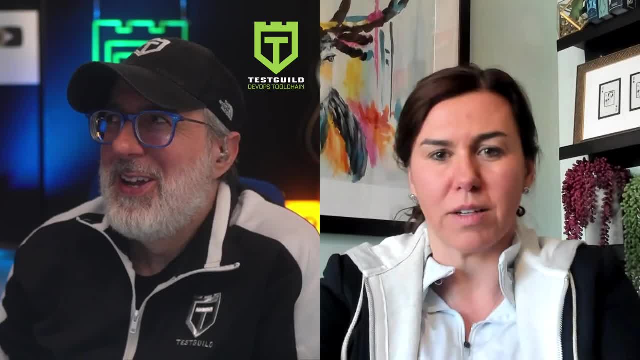 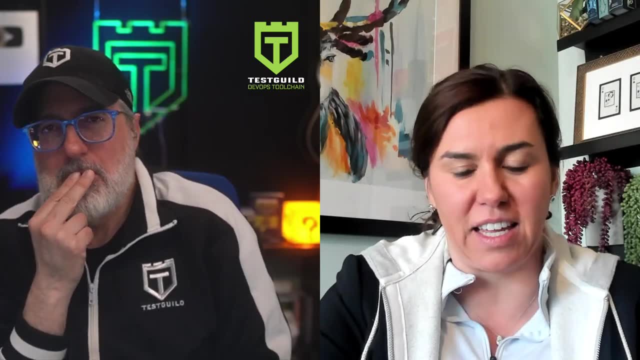 just checkbox. Yeah, sure, But this sounds like it's a little more. you know it could catch a lot of things that you may not even thought of when you were checking in the code Exactly, And I think there was, you know there's been such an emphasis, You know. 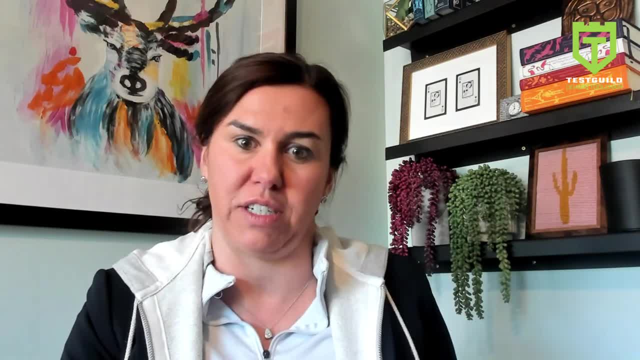 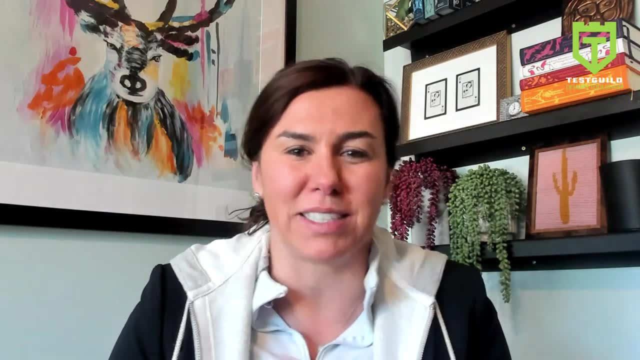 we talked about the scale issue. I'm trying to shift a lot of the data- that's going to be a lot of security- to development, which you know best of intention. you know there's a big company out there that that has done this best of intention but it just creates a mess in a 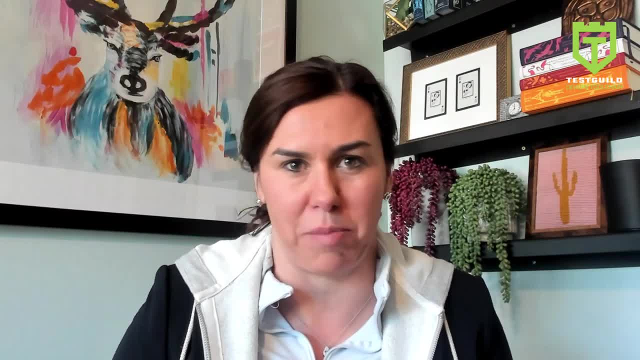 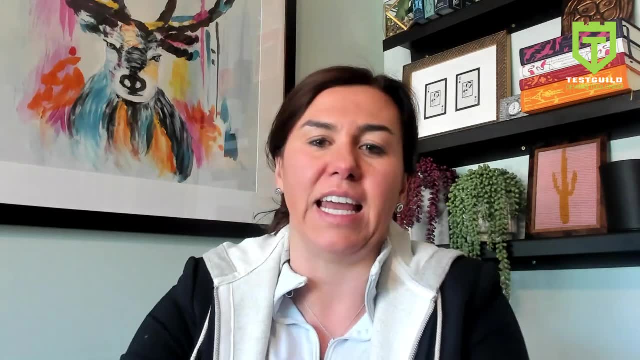 different place, because we're not expecting developers to suddenly become security experts, right. The same way we wouldn't expect security experts to become experts in development, And I think that's where you know we're well past that cultural transformation part. 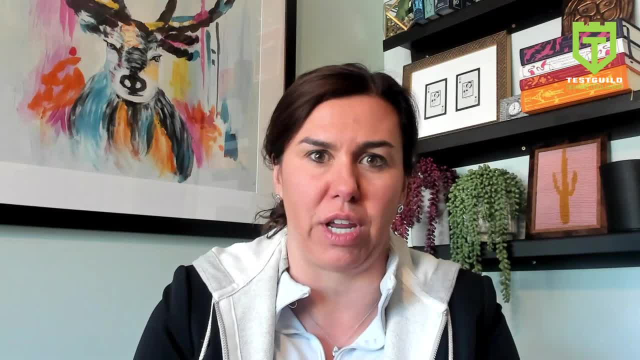 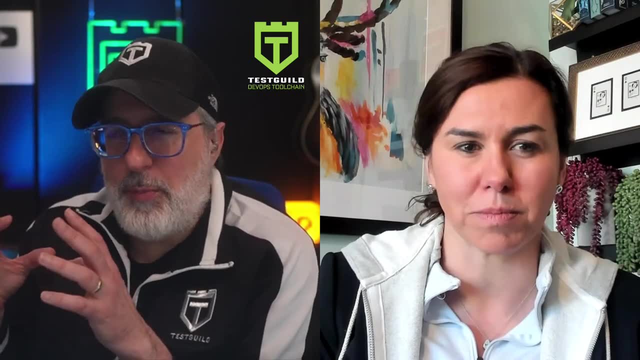 And that's really where our world of application security lives, in the process transformation part, And then we support with the tools Right. So the role of developer really has a lot of pressure on, like you said a lot, some companies that you do everything you do, the testing you do, the security you do. 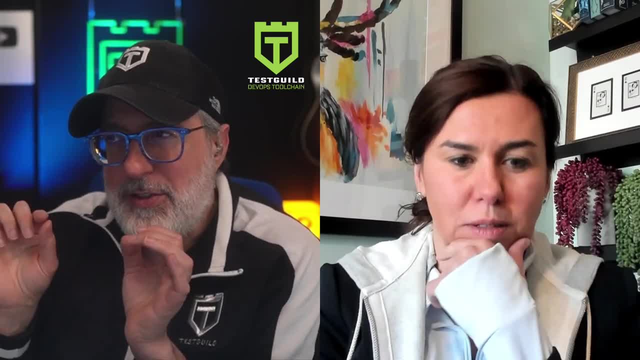 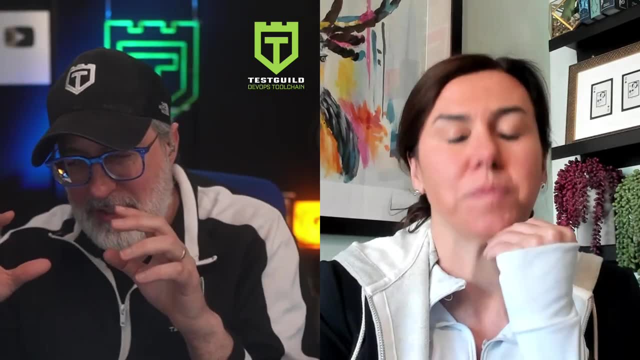 the performance, the whole shebang. So do you see security experts still being involved in the process? Like with your application, do they work with the application, They work with the teams for training, or like, do they do the heavy lifting? They get to become strategic and become really. 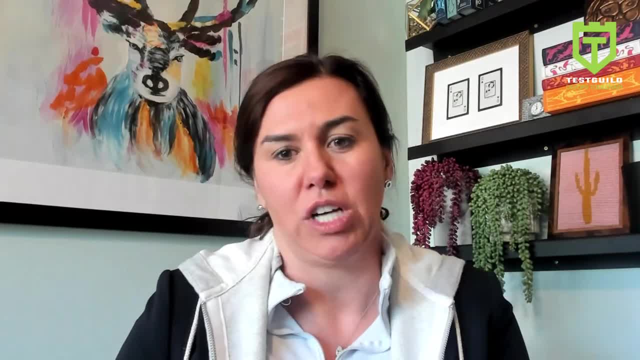 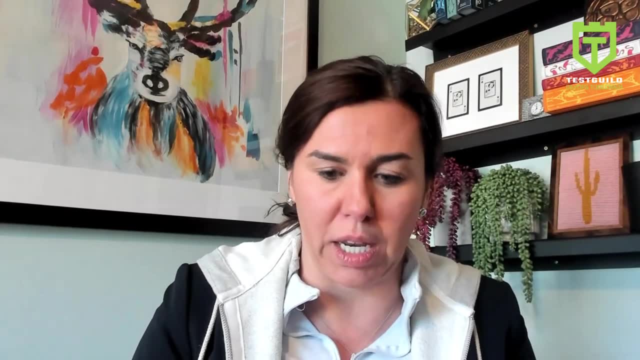 more part of the team, right, And so I think that's a big part of the process And I think we've got a problem. How do we solve it? So there's two ways that security teams get to better interface with development teams, with ASPM. One is, rather than having to wait for your friendly 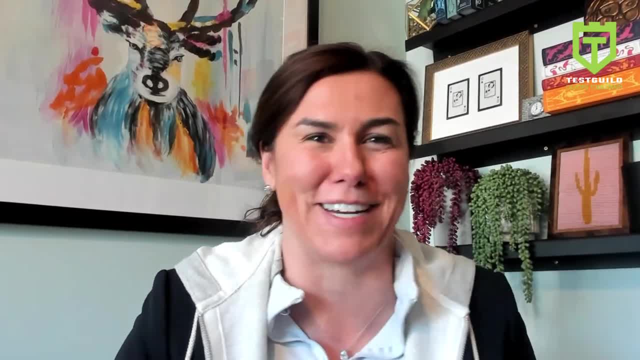 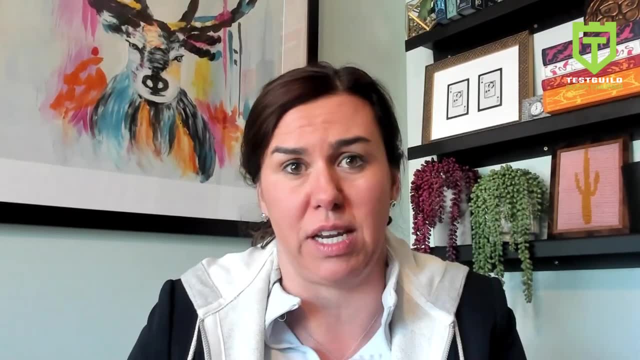 security person to respond to your email or your Slack or whatever. you know, the developer is actually getting that information in real time, And so that's one. So for the security teams, you're actually seeing a huge reduction in the manual work effort. So one of our customers saw: 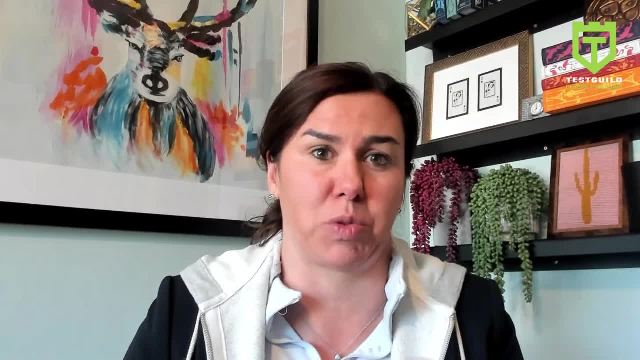 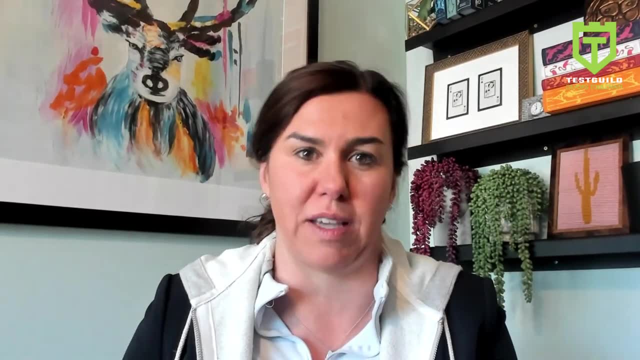 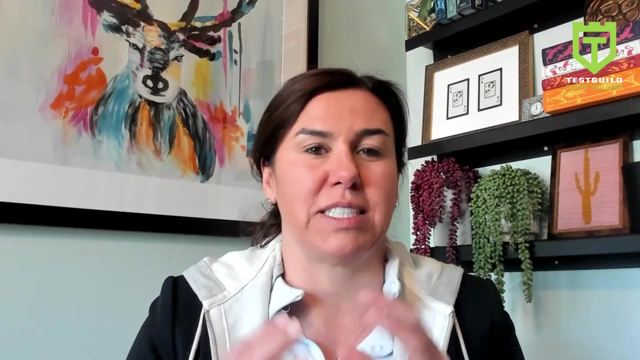 their manual work Flip from. pardon me, their AppSec team's workload flipped from being about 75% manual and 25% automated to being 25% manual and 75% automated with our platform, And the reason the manual work wasn't going away- and they were perfectly fine with it- was because that manual work then became 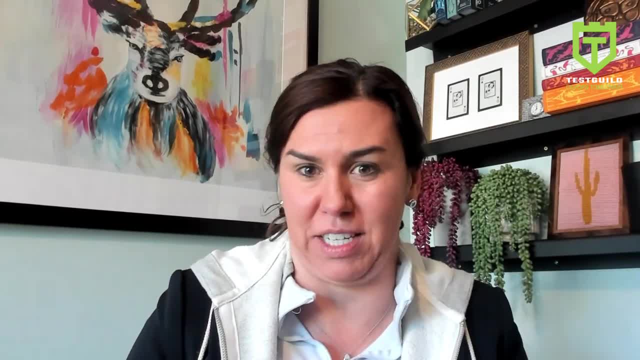 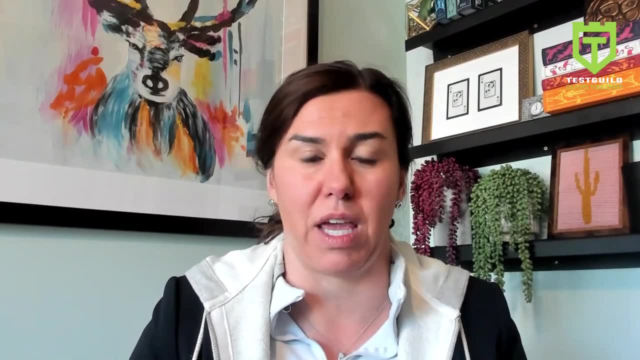 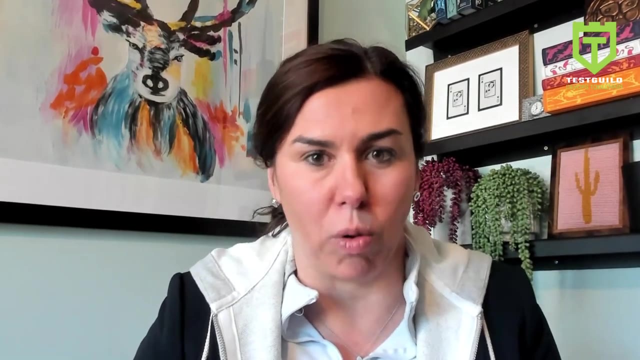 strategic. Are we delivering the best policies to our developers that actually align with how they develop right? I use the example of a policy. might be something like you're dealing with PIA, so you need a 15-minute timeout. Well, maybe it's a bulk import and a 15-minute timeout wouldn't work. 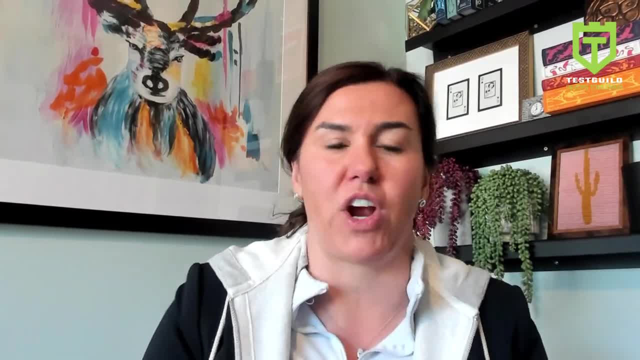 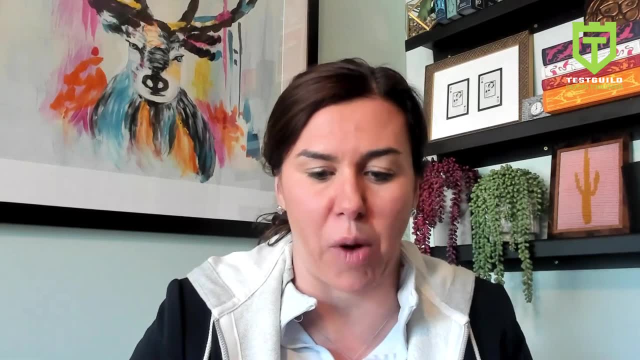 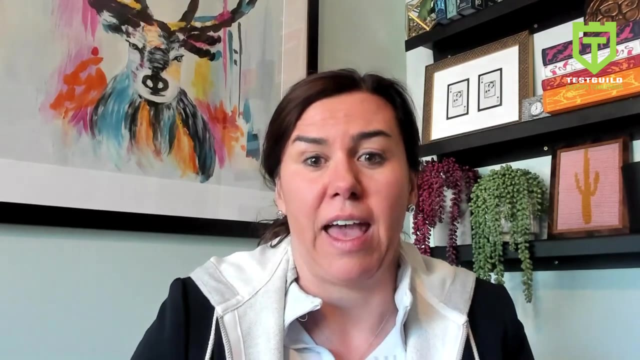 on it right. So let's triage this together and figure out how to come up with a better policy. Or we have come up with a blocker right, And how are we going to work around it? One of our customers uses a library from a well-known software publisher And that customer said: 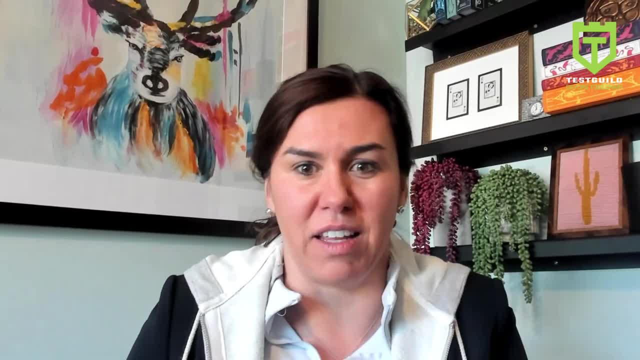 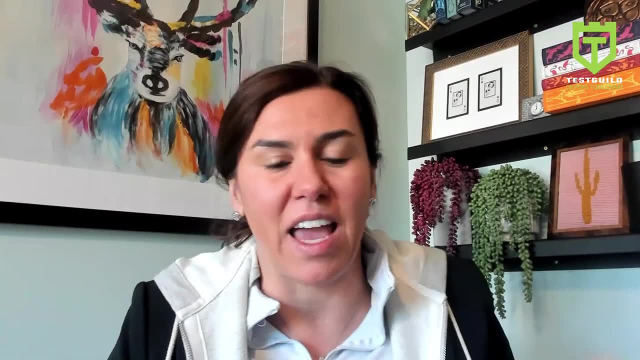 hey, you have a vulnerability, We need you to fix it. And the software publisher said it's not a vulnerability to us, It's not high risk to us, And so they then so the development and the security teams at our customer. 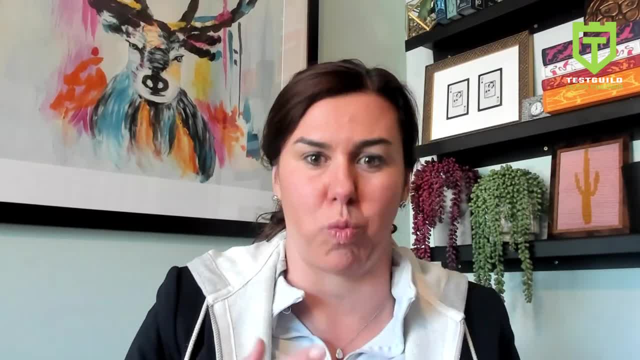 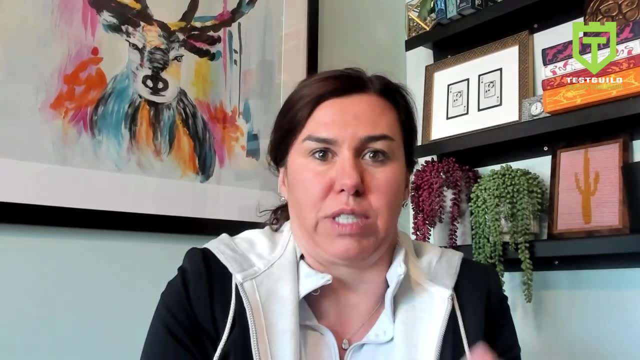 then were able to get together and say: how are we going to manage this? What are the guardrails we're going to put in to do that? And that's again sort of where we step in. We're the guardrails. The security team's got to do the strategy side. Wabi does the guardrails through. 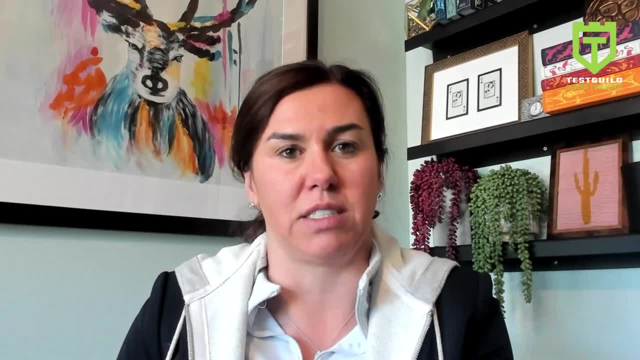 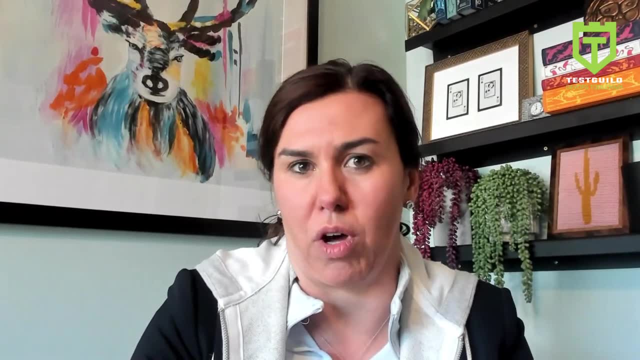 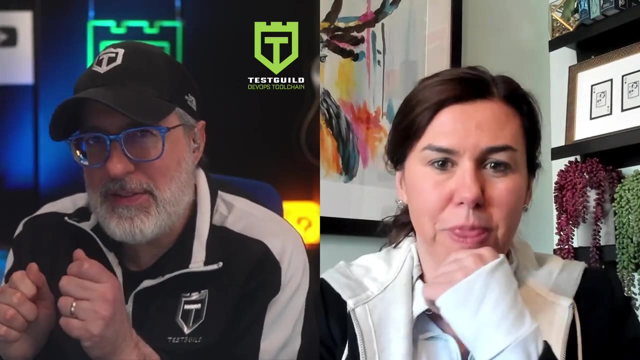 the orchestration and the automation And then development gets the information fed to them And, if needed, they can make the link back to security to be able to work on it together. All right, So what's the current situation with Wabi? if I'm a security expert, Does it mean like they have to manually look through their 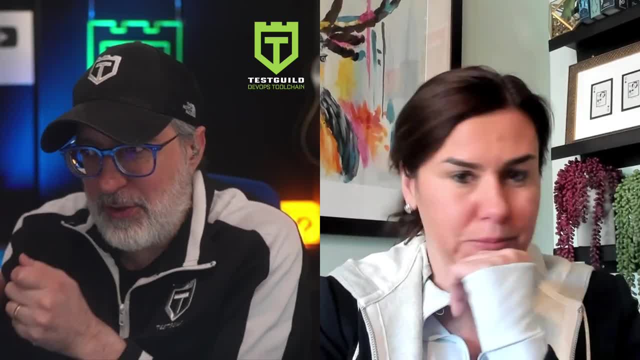 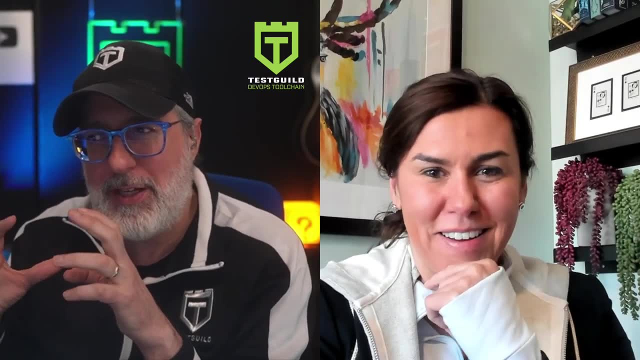 policies. They're manually doing code reviews. They're finding an issue. They're running it over to the dev team. Hey, can you fix it? They fix it, They fix it, They check in, They go back, They review it. Is that the manual type of workflow that this replace? Correct Right. 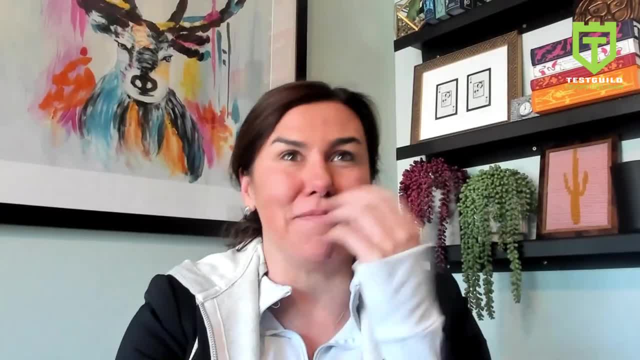 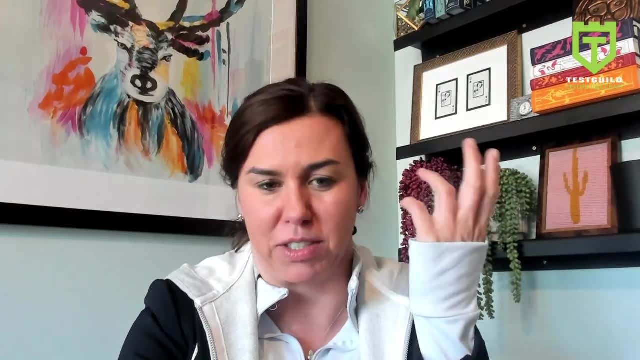 That's if they can get there in time. I mean right. Much more tactically right. You get- and these are in well-educated DevSecOps teams, right? One of our customers develops essentially DevOps software And they said, hey, my teams are actually very aware of this And I get 10. 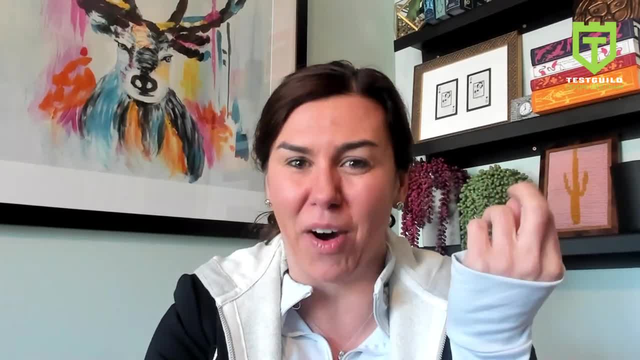 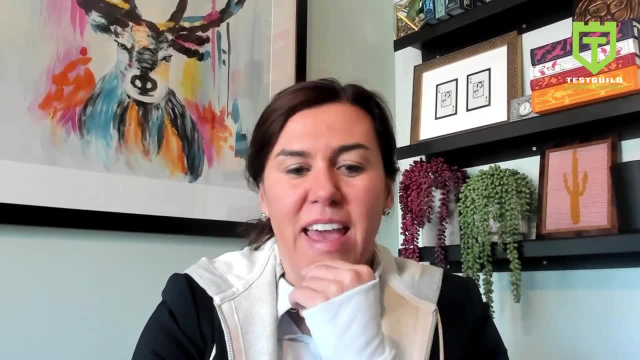 emails a day saying: is this the test I need to run now, Or do you need me to fix this vulnerability Right? That's a bunch of time that he may or may not have, And that's exactly what's happening today. I could pull up a web browser and I could pull up a web browser, and I could pull up a web. 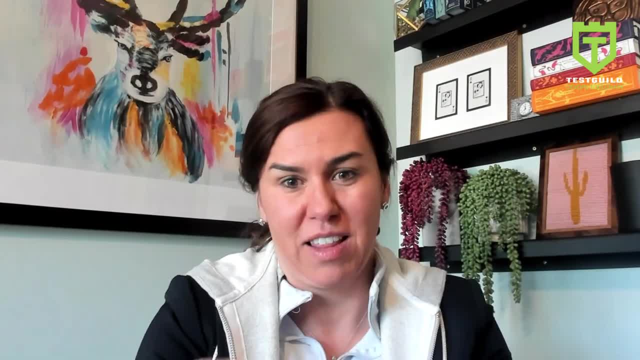 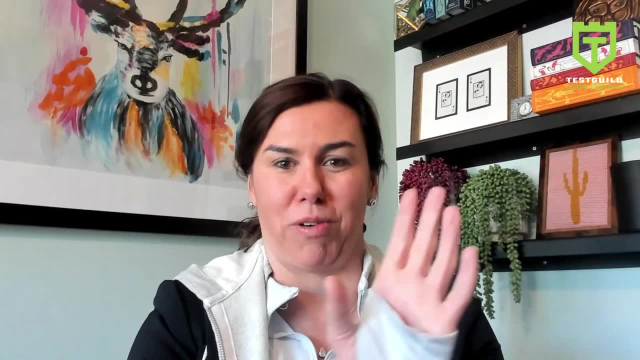 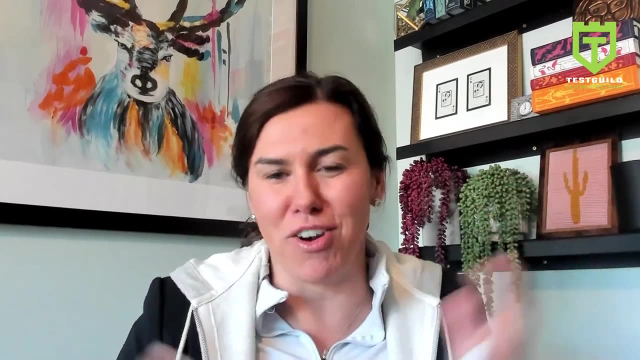 browser and I could pull up a 12 sheet workbook that one of our customers uses or used that. that was the security code review checklist. before they could do it And and want to know what it did, It referenced a bunch of thick PDFs that nobody knew what it was and what does it mean for me in this? 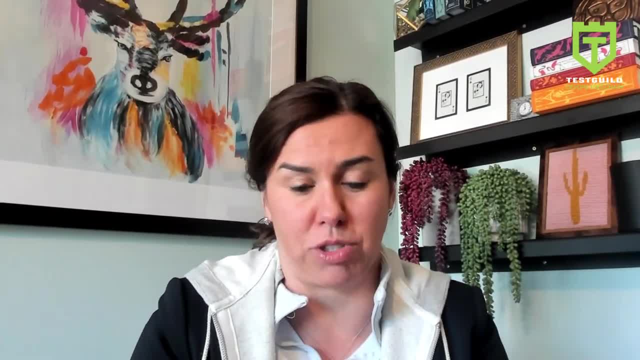 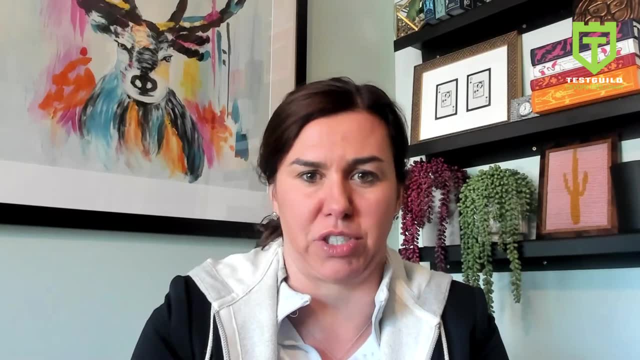 moment, And that's where we're really trying. We, we try, and we do take the the need for, for expertise out and we spoon feed The information: the right place, right time, right person. And so that way, as things change, 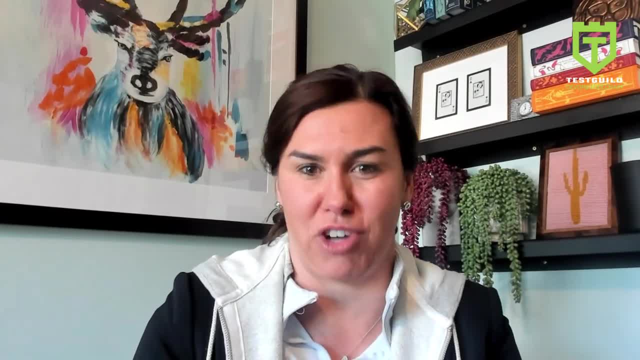 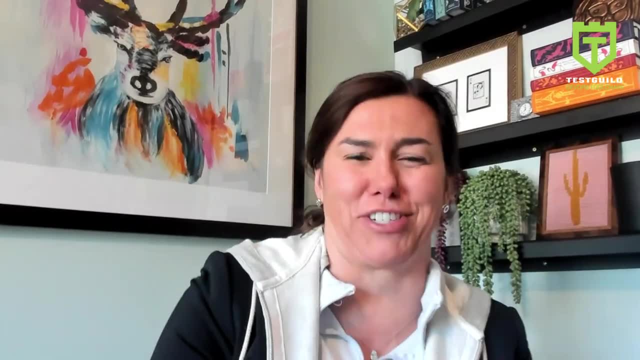 you don't have to be, not that we won't all still always need security training, but you don't have to be reeducated in what the new policy is. But yes, what you described is exactly how application security happens today without WAPI. 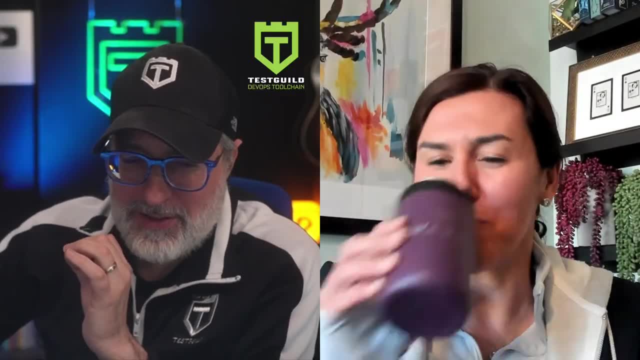 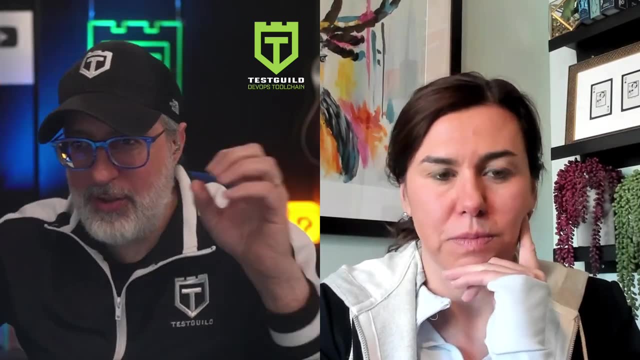 So this might've been a bad implementation, but when I used to work with and we had security scans, there'd be like a lot of false positives. And then there's so many, so much information, so many things that people didn't know like. 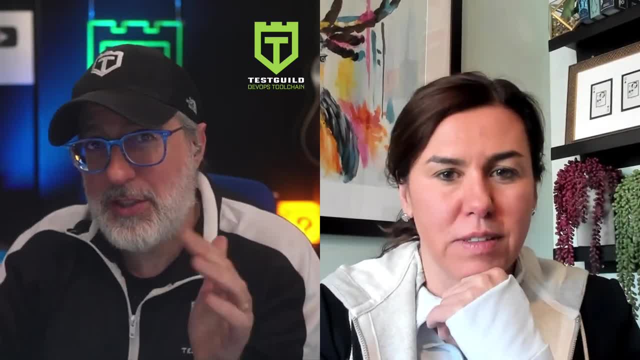 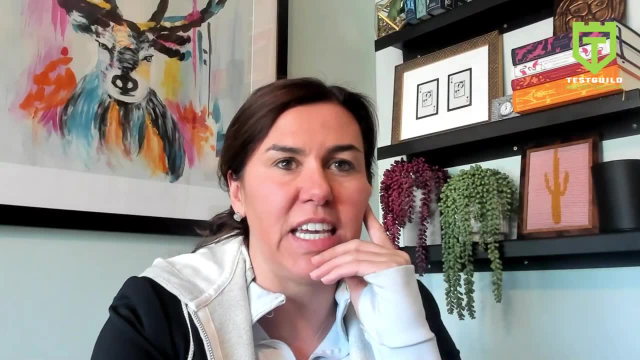 what to focus in on, what was real, what wasn't, and they would just ignore it at some point. So this solves this as well. I would think right, Like, how does it solve this issue? And that's a key, you know, I mentioned it earlier- If we think about application security, 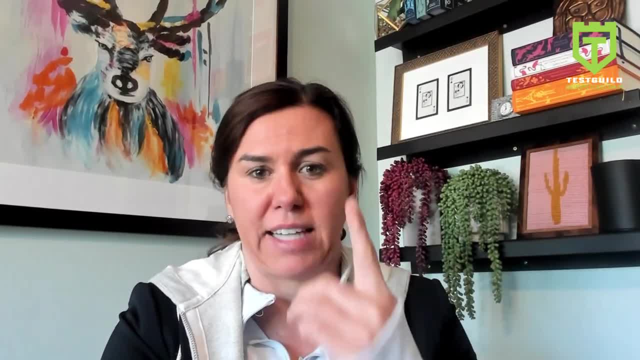 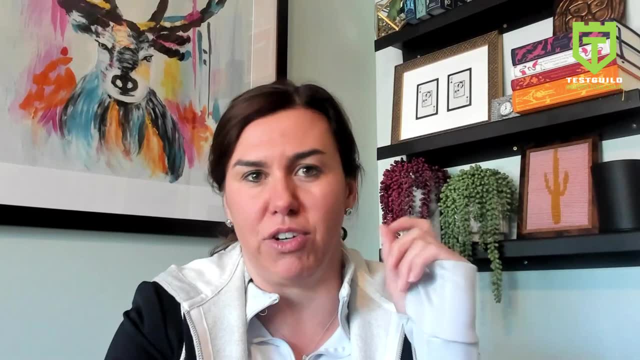 posture management. it really deals with three realms, and that's the realm of vulnerability management, which is really, if you just think about it, a specialized kind of tech debt. You're starting to see the new buzzy term, risk-based vulnerability management. And, again, 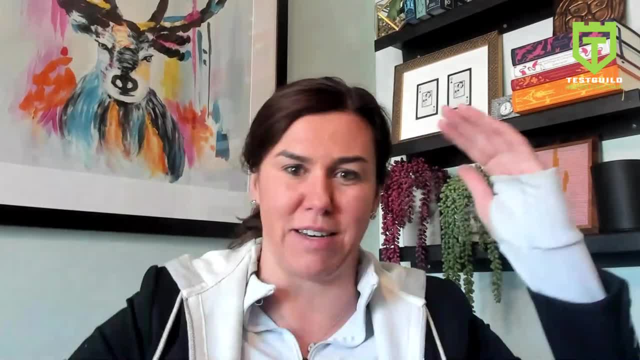 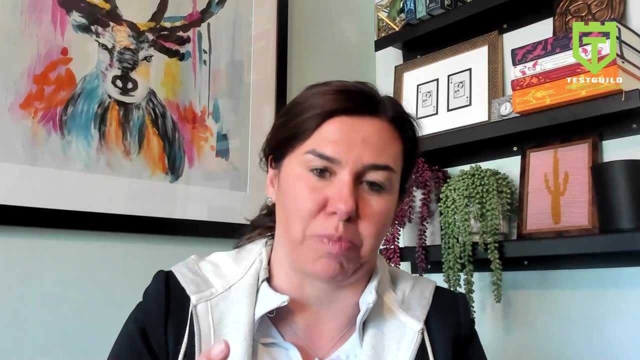 that's just criticality Plus severity. What do I need to fix And in what order do I need to fix it? And that we absolutely do. but you've got to have it as part of the whole puzzle, right? Because if you're just doing vulnerability management like if you're just grooming- 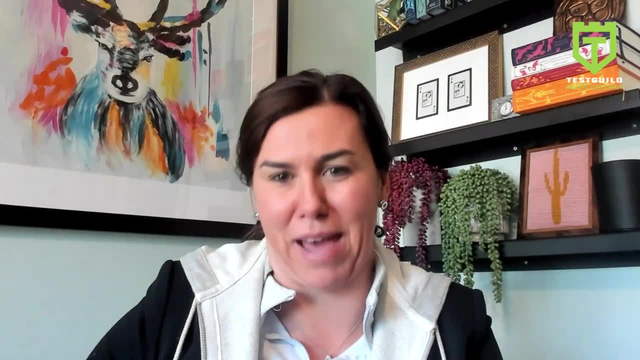 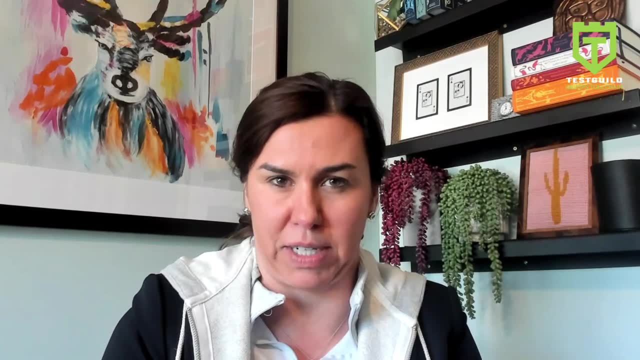 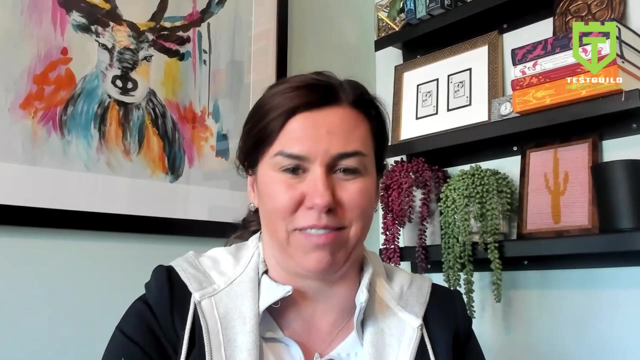 a backlog in a closet by yourself, right. What does it matter? And that's you know that vulnerability management- the big thing that people have accepted, which was tough and is tough in a lot. most organizations that are still building exactly what you described. that that will feel very normal to a lot of people in your 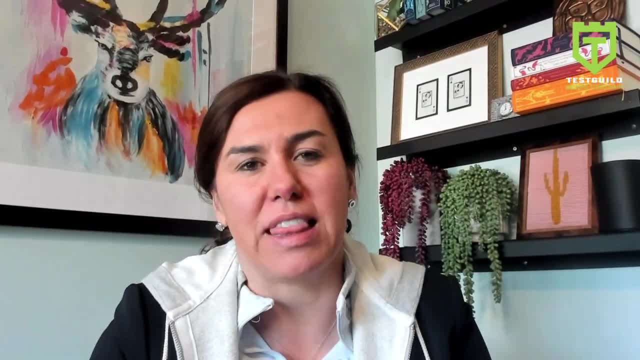 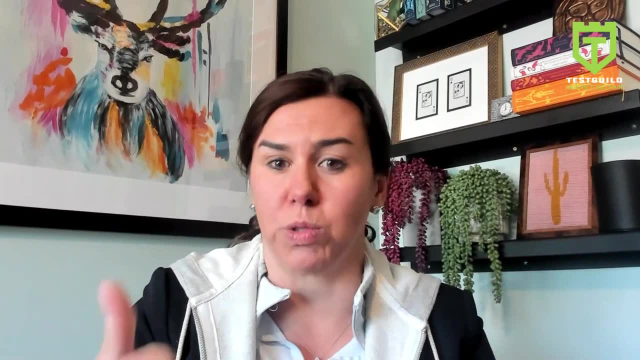 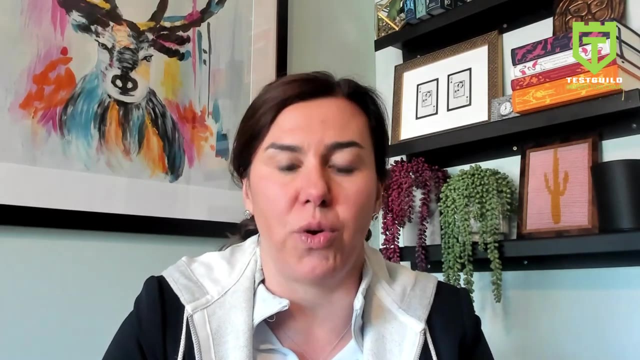 audience. You know they were getting all this data thrown out at them And, first of all, it wasn't aggregated it across tools and time. And the second thing, it wasn't contextualized for that company or for that application, And so you need one record right. And this is how Wabi approaches. 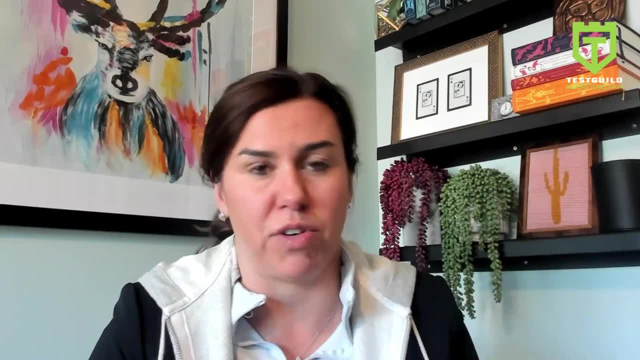 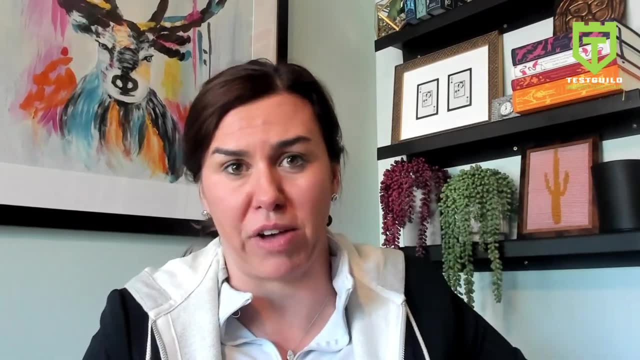 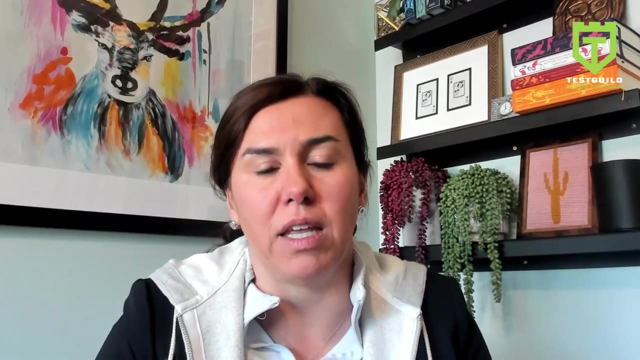 it. We have one record, We can roll it up and even see the vulnerabilities and different assets, because you may even have a shared asset package, a shared asset between a low value application and a high value application, And that would change the rules that you'd want to apply, And then, across time, and then we reprioritize it to. 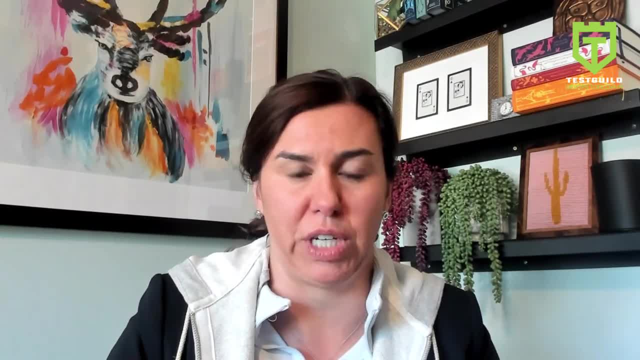 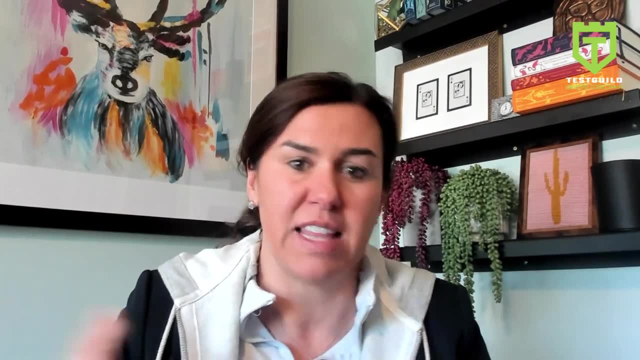 say, hey, we actually care a lot about this vulnerability and that needs to go in the 5% that we're going to fix this month. And then there's 10% to maybe even 15% that we can fix later. So what are the SLAs around that? And then what about that 80% that we just need to sit and 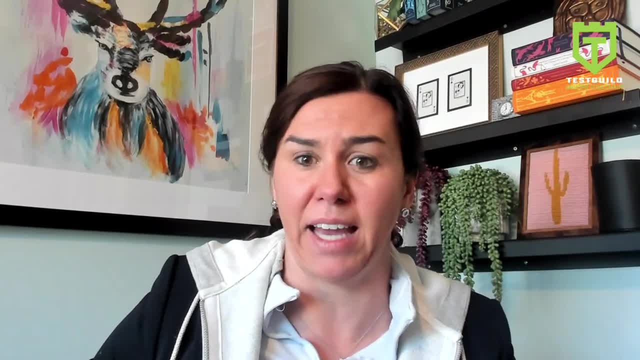 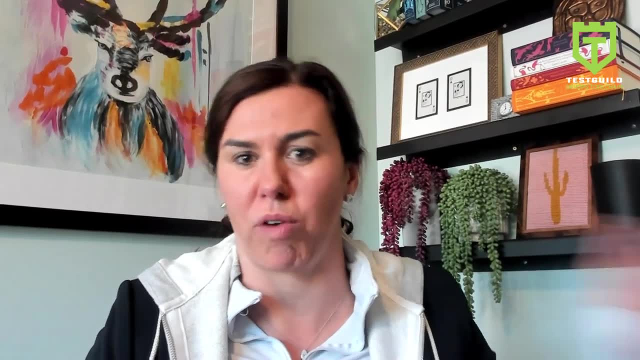 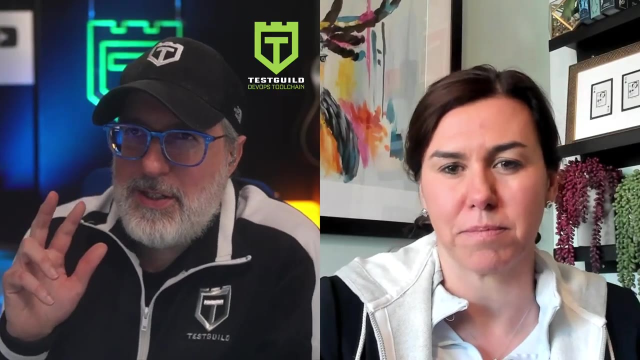 monitor so that it doesn't become something bad and maybe there's a different future rule, but that actually never needs to end up back in the developer's backlog, because we're fine, accepting that risk, because we can't fix everything, Love it All right. So here's a long question. I don't 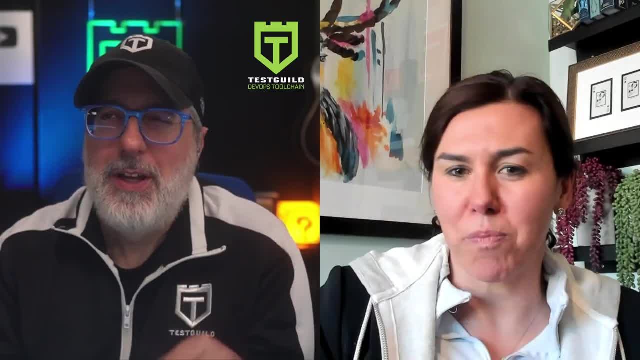 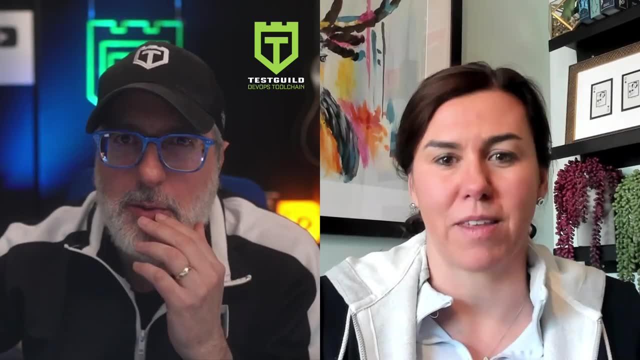 even know if it's going to make sense, but let me try to unravel it. I run a news show on automation and DevOps and I've been seeing a lot of news recently around the security, like with the White House. I think they unveiled a fiscal plan recently and it was like $13 billion of injection. 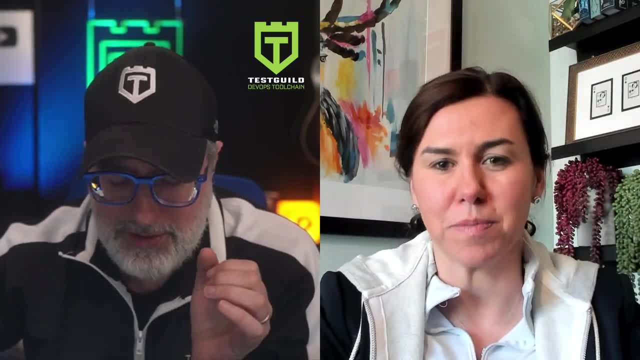 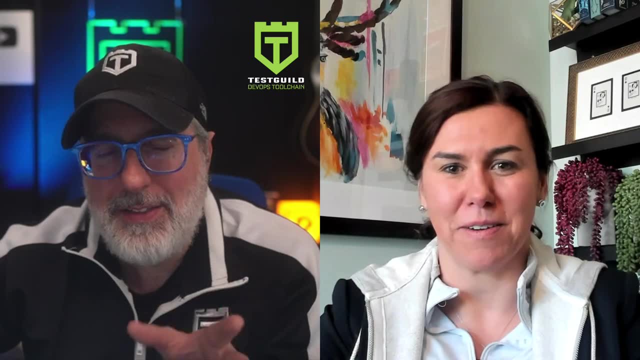 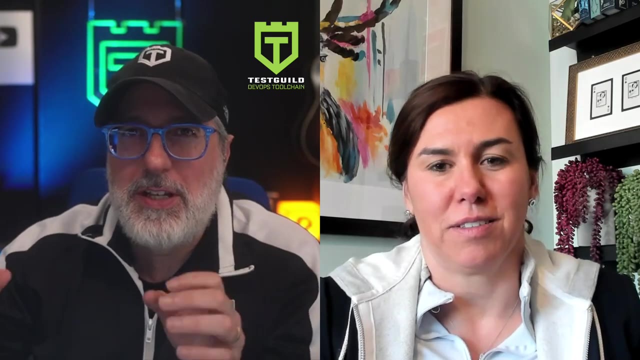 to the federal cybersecurity budget, And they also released something called a back to the building blocks report, where they said the burden of cybersecurity should fall on the shoulders of tech companies and the federal government rather than individual users. And on top of this, you mentioned that Gartner mentioned ASPM as a transformative. 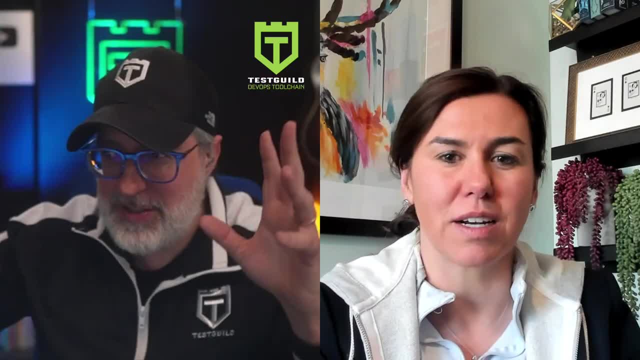 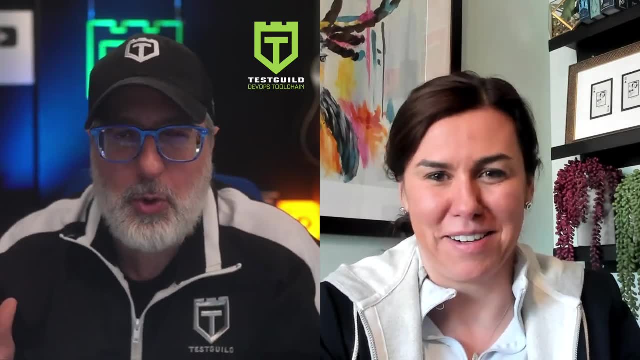 technology coming into play. So is this a convergence of like? is this where we're all heading, And is this why people should really pay attention? now, Like every time I see the government releasing any reports, even though they say they're not going to, I feel like I'm 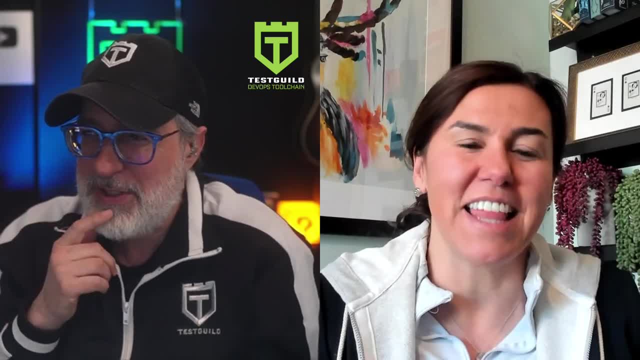 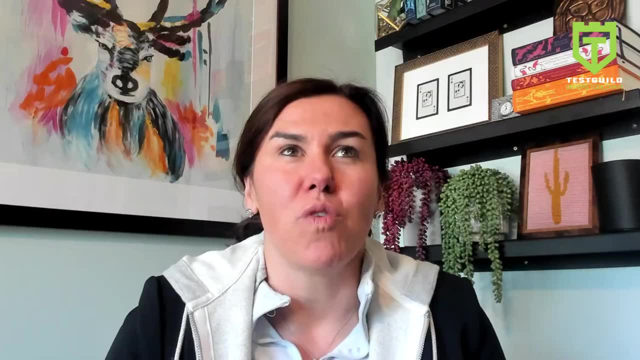 going to start poking their fingers into it And that's going to cause companies to really take notice. This one I have not minded too much, So I'm going to split up that question, You know. first, one of the problems of application security is that it's always been a little 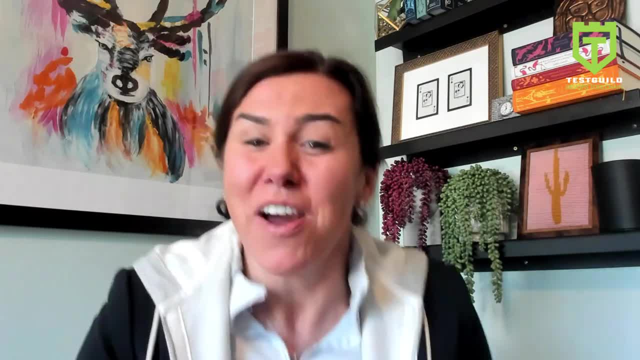 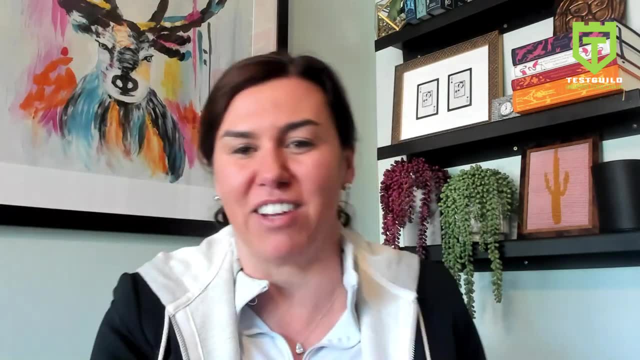 right, It looked too develop-y to be security. right, Because it's proactive. It's about the process, And in development we set a process because that's how we get things out and make decisions about it. And then it looked too security-ish to be development, And so it's. 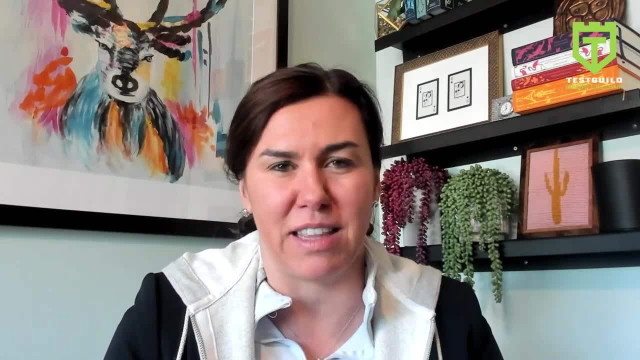 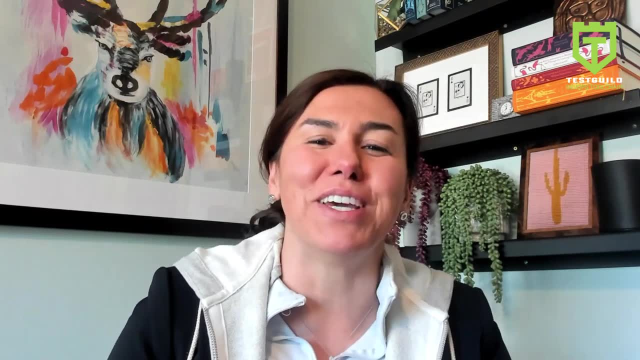 sort of been out on its own. But the harsh reality that nobody ever talked about- and why I'm glad it's getting so much spotlight now, even if it does mean one more government report, you know- is that nine out of 10 breaches begin due to defects in code. You rarely, rarely hear about it in the news reporting because it'll be something like ransomware. the hackers, you know, did this kind of infiltration- MITM, whatever it is- And but what it was was that defect in the code, that vulnerability that wasn't fixed or wasn't. 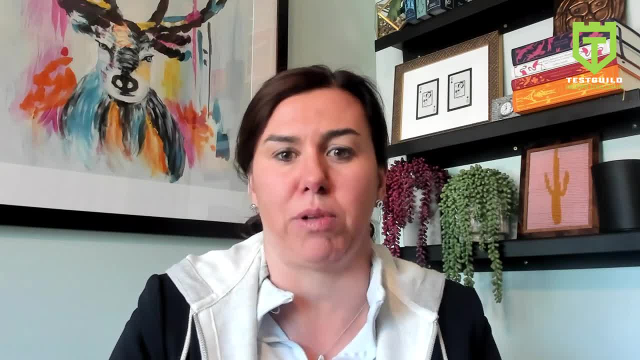 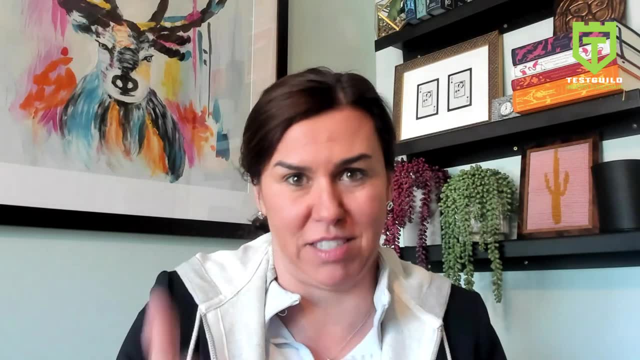 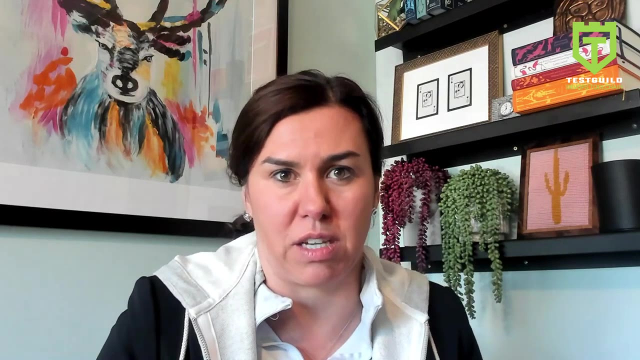 found, provided the entryway for them to be able to execute on their attack. And so now application security as the building blocks. I actually thought they did a phenomenal job with this report, as the building block of security is where we're starting to see this convergence that I say. 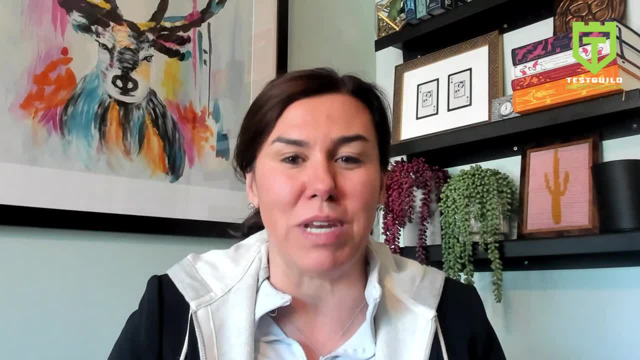 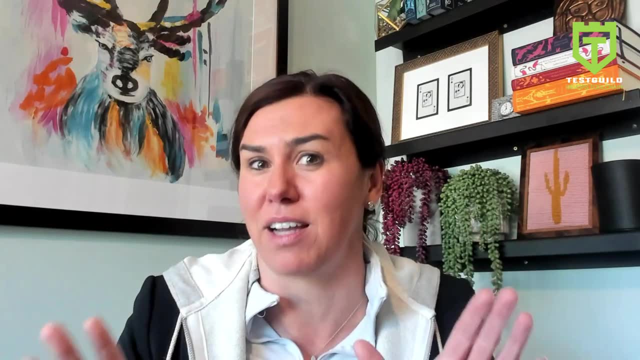 application security is all security right, Because if you need a taller wall and a deeper mode- and this is a little bit where they get into- the burden falls on the tech companies because, remember, every company is a tech company today, even the government in its very 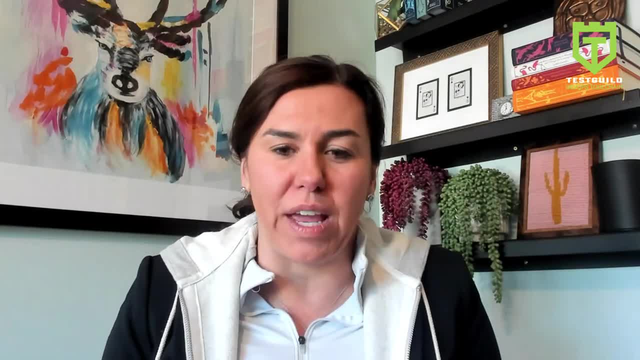 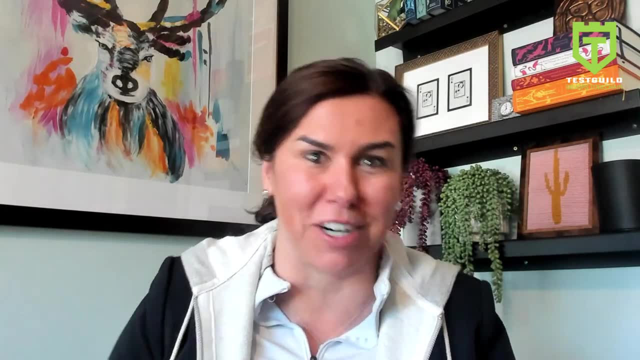 word ways And and you know, and, but if you want a taller wall and a deeper mode, right aka firewalls and you know, and better network security and and AI- a part of me- API security and AI security and stuff, you've got to work with the development. 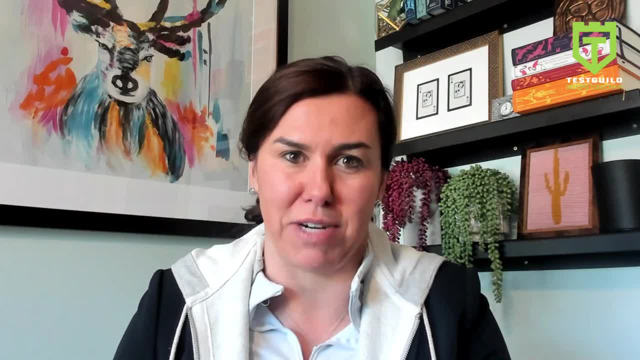 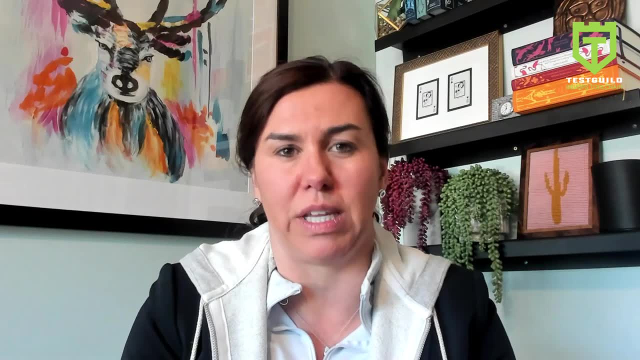 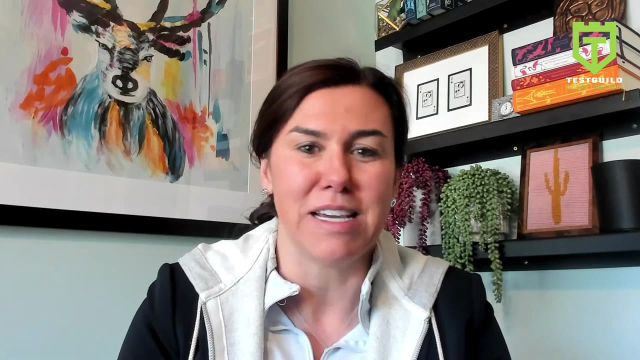 team to execute that right. There's very little security nowadays that exists without collaborating with, with development, And that's really why you're seeing application security posture management become this transformative. you know hot button in technology that people want because you can't bring together all those pieces And you know I go back to sort of our 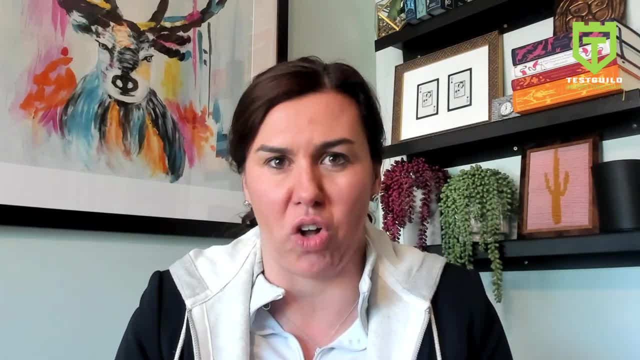 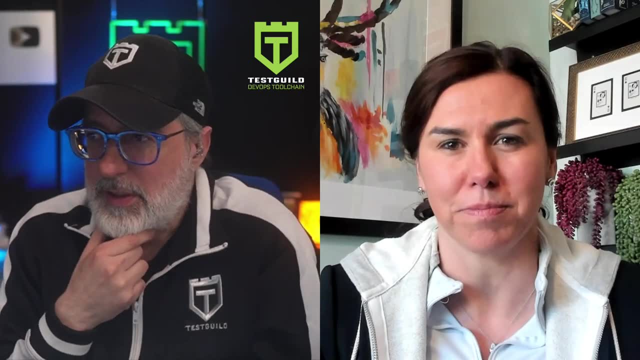 starting point, conversation about DevOps. At the end of the day, all of this is just good development, because it's about good collaboration and breaking down silos. Love it, And you know, with the speed of development nowadays, this is almost like. 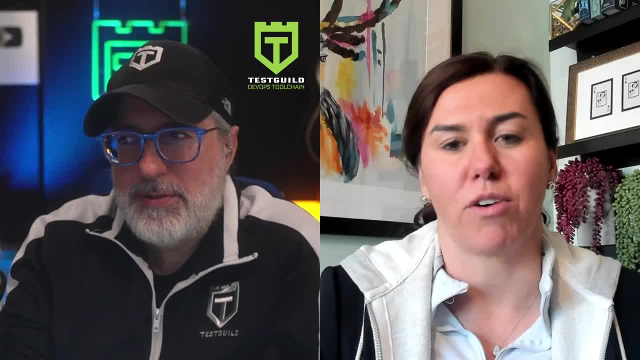 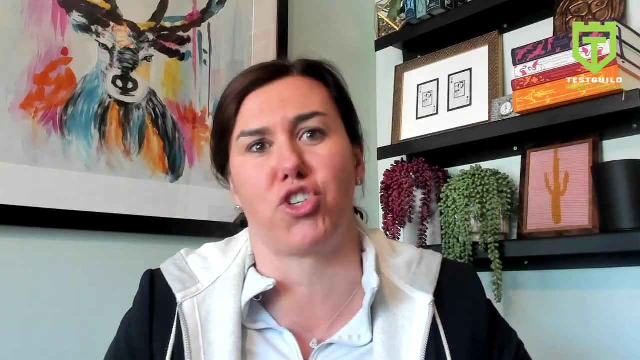 automating the gap between developer and security almost sounds like Correct, Exactly Right. We're not expecting, nor should we, developers to suddenly start doing different things. right, They've got good workflows. those will evolve as development evolves. Same with security. 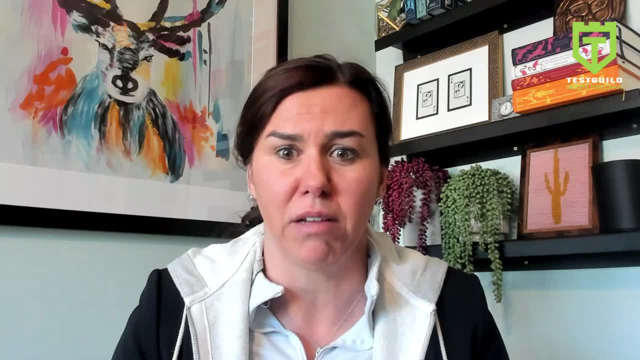 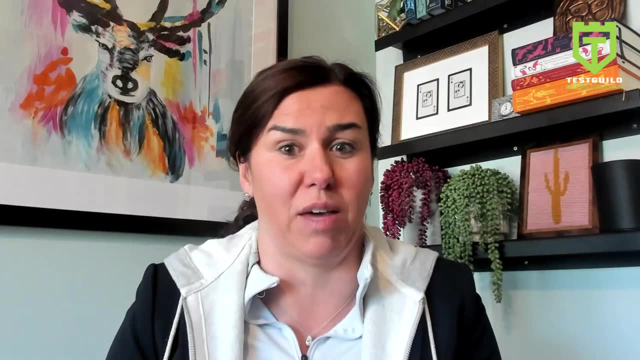 They've got their own workflows right. Developers crave autonomy and information so that they can execute on that autonomy And security. professionals crave accountability. Did you do the thing that we're supposed to do to make us safe? And so we. you know this. this has always been our philosophy. 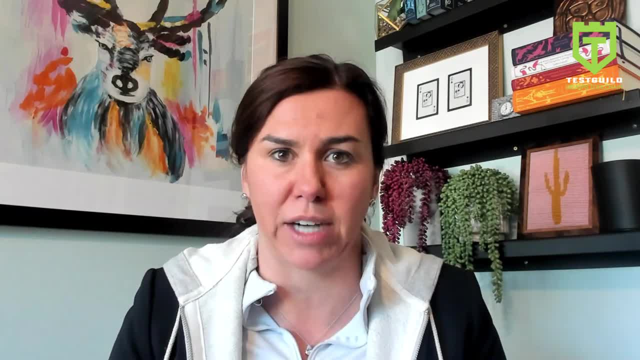 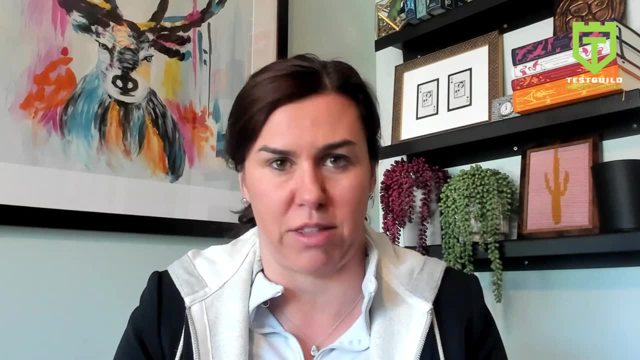 and our pillar around you know how you actually integrate security into development is: let everybody do their own thing right And the way that they want to do it, and find a way to translate the two into each other, And that's that's you know, that's you know, that's you. 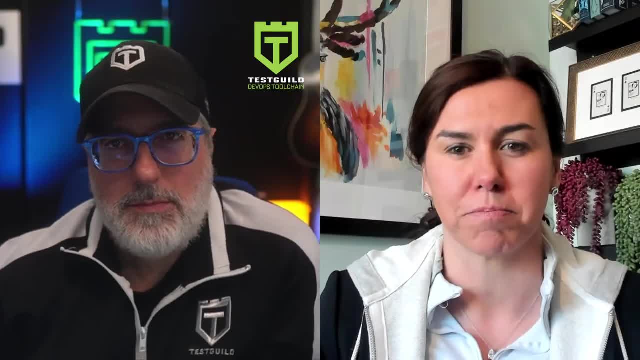 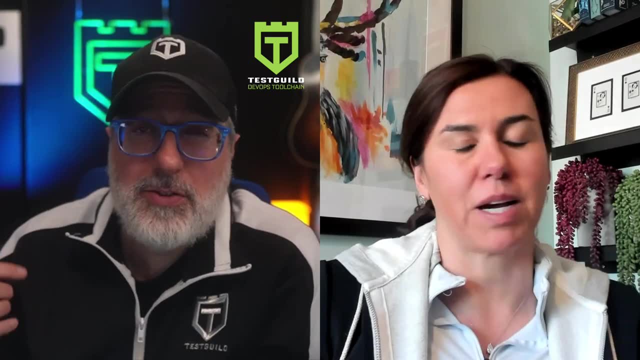 know that's really the future of how we address this problem. Nice. So if someone's listening, Bobby like I have to check this out. How hard is it to integrate it into existence systems? A lot of times I think I used to work for healthcare insurance companies. 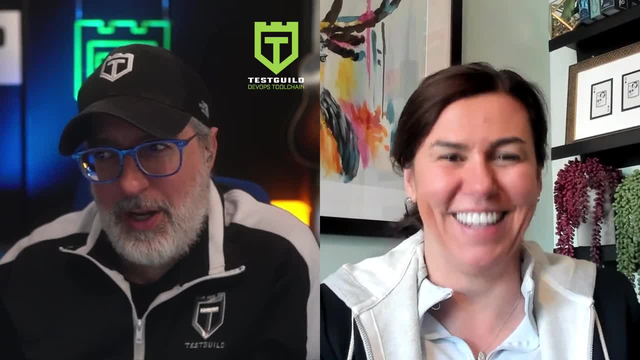 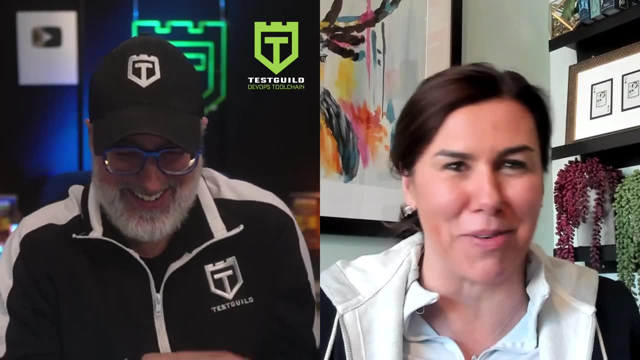 older companies that kind of have a legacy things like: how, how do you, how hard is it to implement? It's interesting. You bring up the legacy things right. Don't worry, We're a hundred percent cloud. We know, one day I guarantee you have a server sitting in a closet. Absolutely Yes, It's. 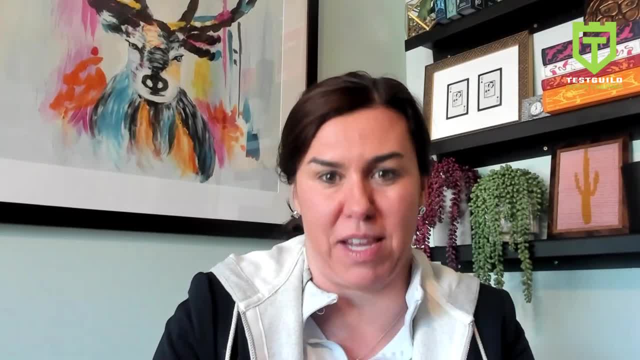 it's something that we actually said. if we're going to make this work right, we have to make it very easy. So obviously you know we're API centric, but one of the things we did because we realized very our customers being very large: mid market, fortune 500, some in DOD, you know they have that complexity that says, Hey, I've got this system. you know, don't worry, we're going to sunset it one day. We actually developed an agent that allows if somebody needs to connect to an 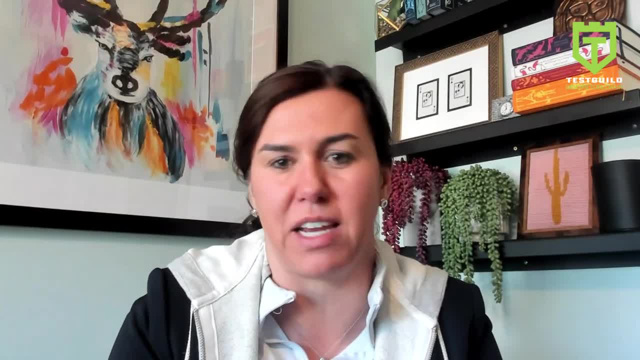 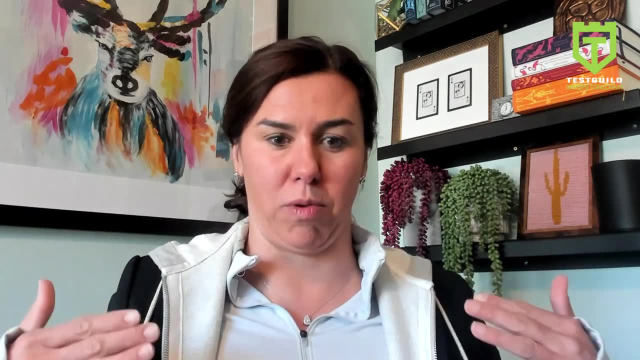 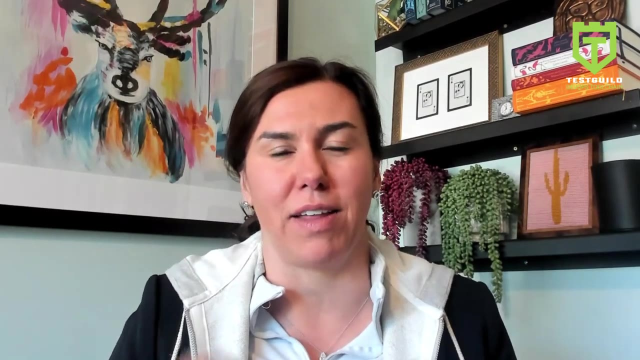 on-prem system, right, Sometimes it has to do with sensitivity of data and other things, And so for us, right, the analogy I like to use about Wabi and how we work is we rely on those connections, but what you want to connect to is going to change over time, And it's kind of 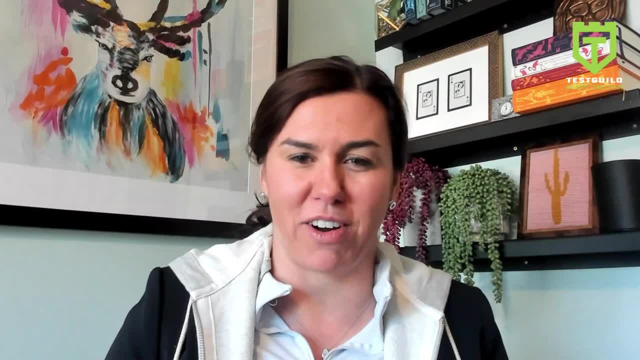 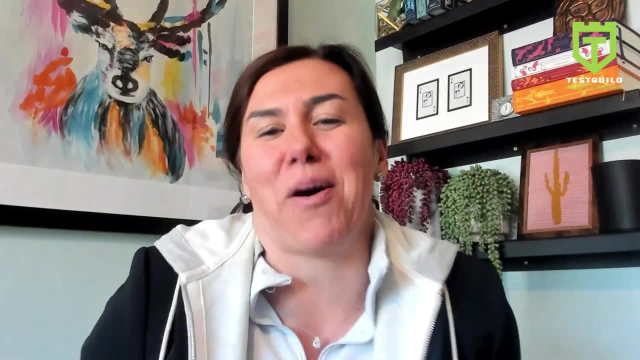 like if you remember pictures of the old telephone operators when I'd call and say, Hey, I want to be connected to Pennsylvania. three, four, five, Hey, and they go. okay, sure, Hold on a second. That's how we were built: to be able to say, Hey, look, I'm actually at a different phase in my development, Trans transformation, And now I'm using serverless and I want to connect to a serverless security program. Can I do that? Great Right, We can build an integration for it if we don't already have it. And and now you have that serverless or the other side could be: Hey, we're going to serverless. 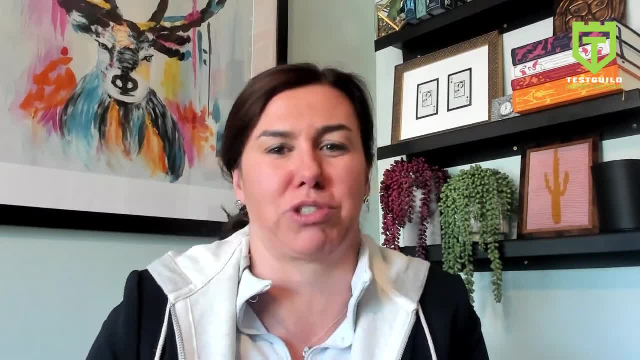 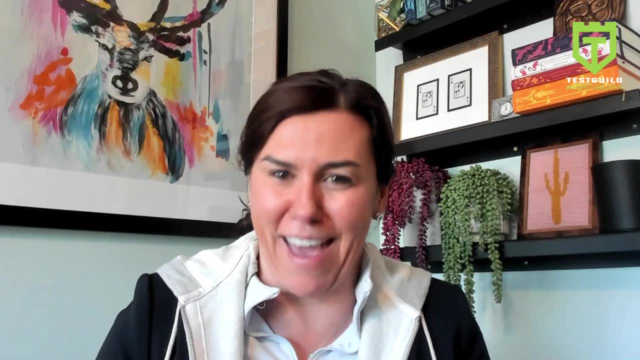 and we just need attestation. right, We just want to know, right, Cause we're still experimenting on cool Wabi can do that And it's it's the recognition that everybody is a special snowflake and and and right And your program. 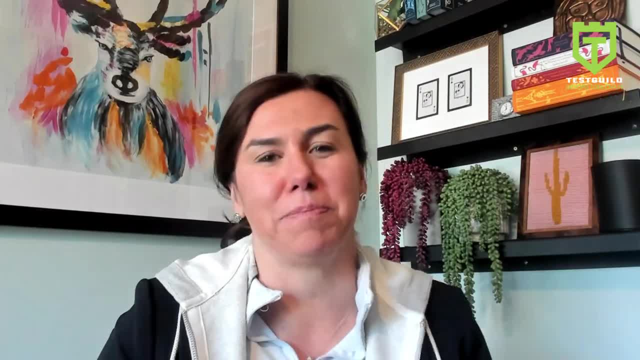 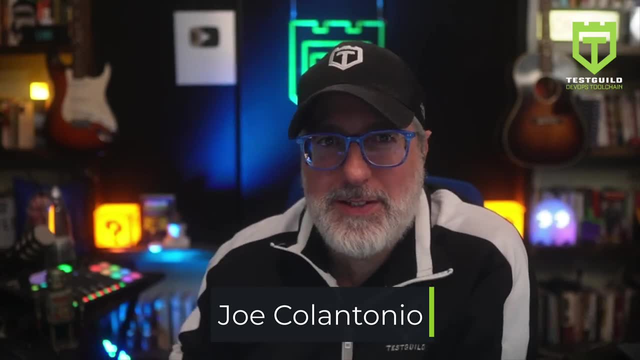 It's going to be different and we've got to be flexible to roll with that. Great Okay, Brittany, before we go, is there one piece of actual advice you can give to someone to help them with their DevOps security efforts, and what's the best way to find contact you and 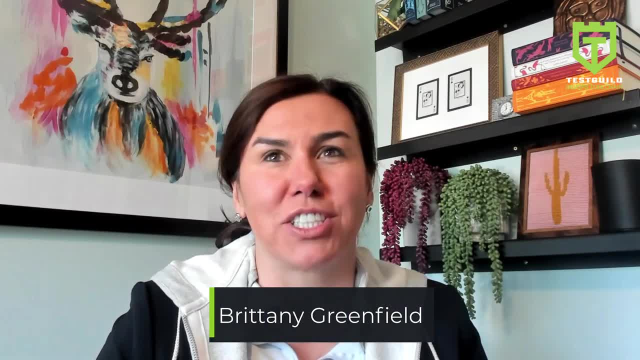 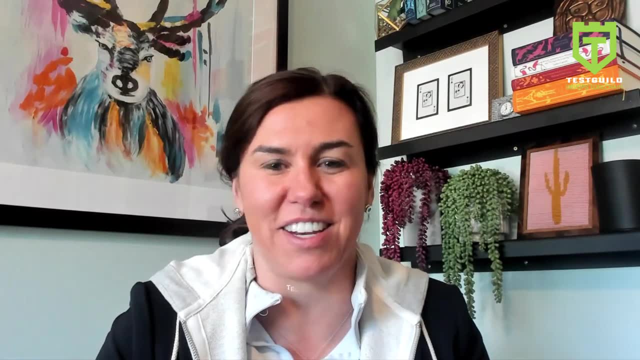 learn more about Wabi Yeah, The um actionable insight. I would say: pick up a phone and call an application security manager. Um, I really mean this and I don't mean to sound all Kumbaya, but if you're a developer or in a development organization, 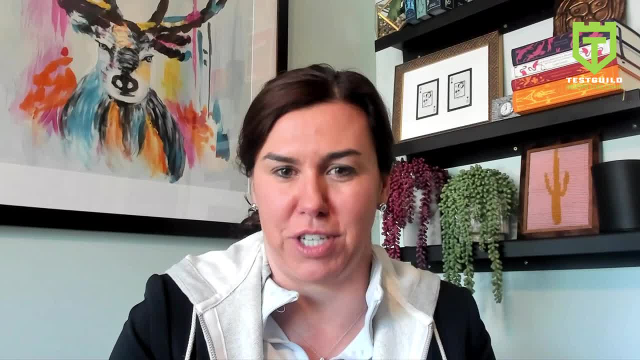 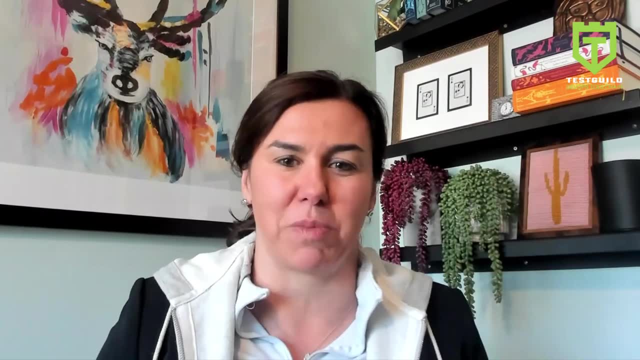 ask them what they are trying to achieve with their application security program- No different than what we discussed here, where you said: I think of application security, I think of testing. It's such a much bigger puzzle- and ask what you can do to help that. 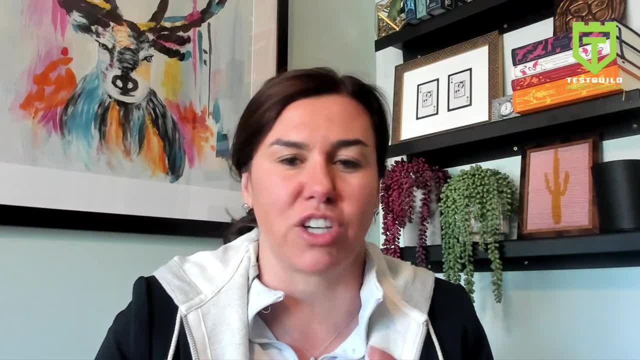 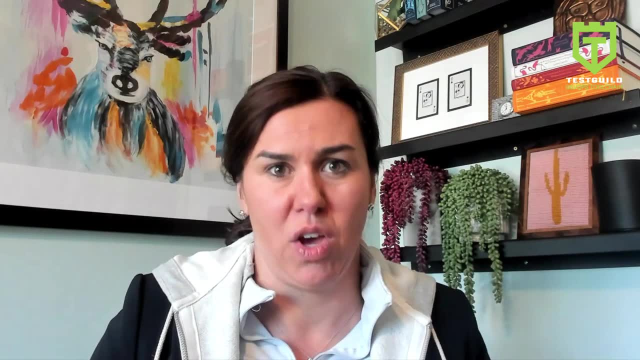 That's the one actionable piece of information I think I can give, that that's going to move the ball forward a lot faster. Um, because right now both teams are getting inundated with too much data and they don't have the context to turn that into information. And when?